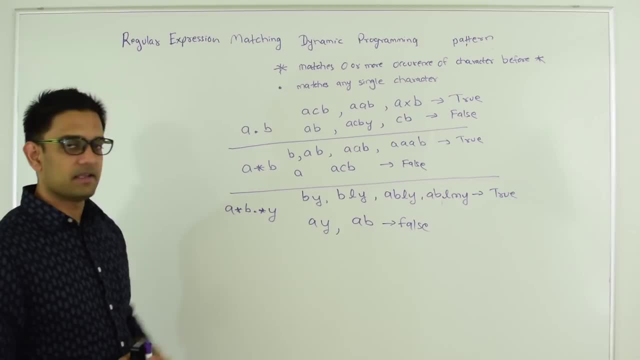 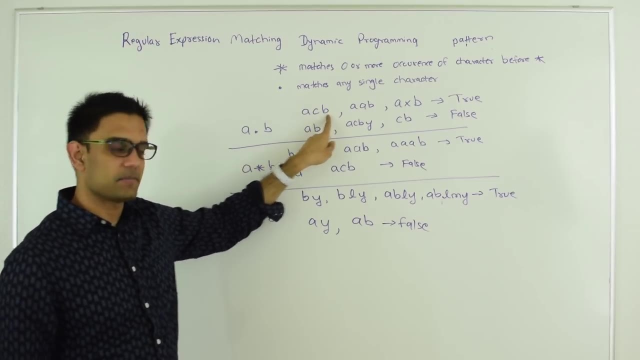 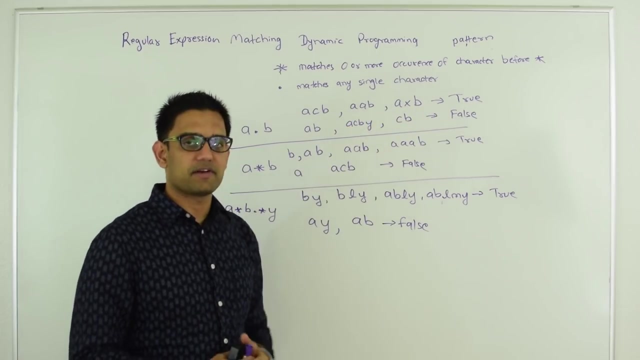 explain this with example. So a dot b. So here we can have any single character between a and b. So for example, if my text is acb and if my pattern is a dot b, then that is a regular expression. match aab, axb. all of them are regular. 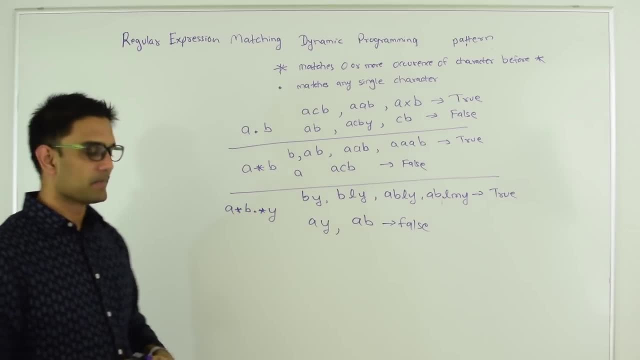 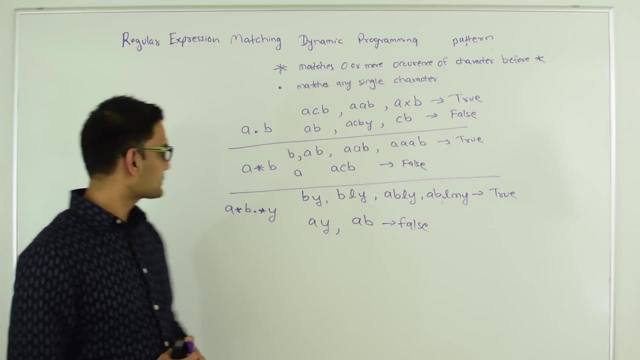 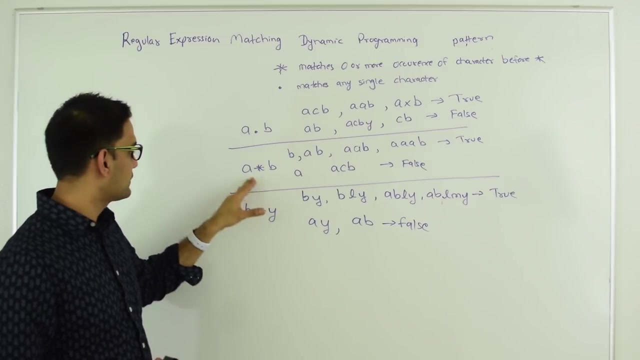 expression match As long as there is any single character between a and b. On the other hand, ab, acby cb are not a regular expression match with a dot b. Another example: a star b. Here what we're saying is we can have zero occurrences or more occurrences of a followed by b. So if 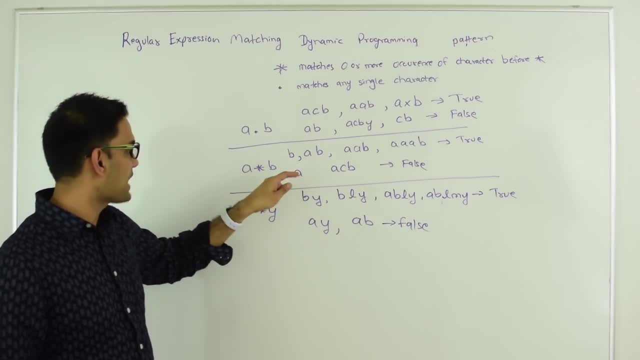 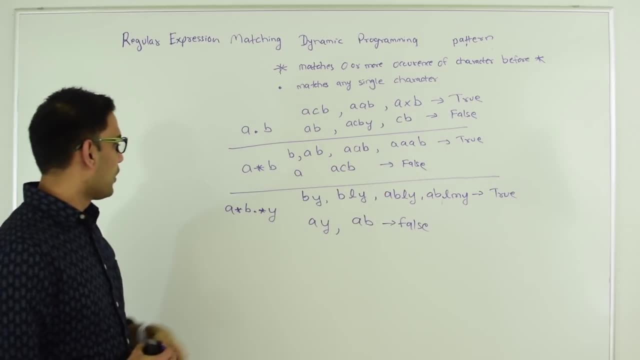 my text is b and if my pattern is a star b, so that's a regular expression match because we can have zero occurrences of a. Similarly, ab, ab, aab- all are regular expression match. On the other hand, a is not because we need one b at the end. Also, acb is not a. 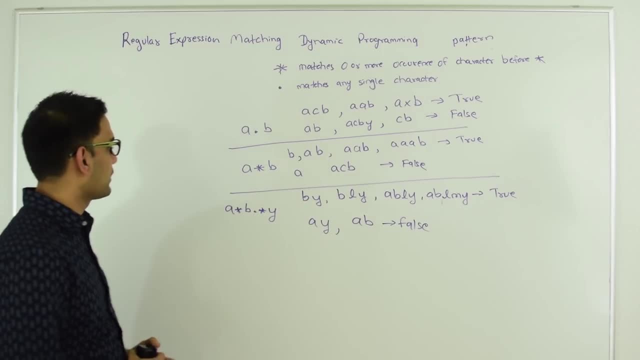 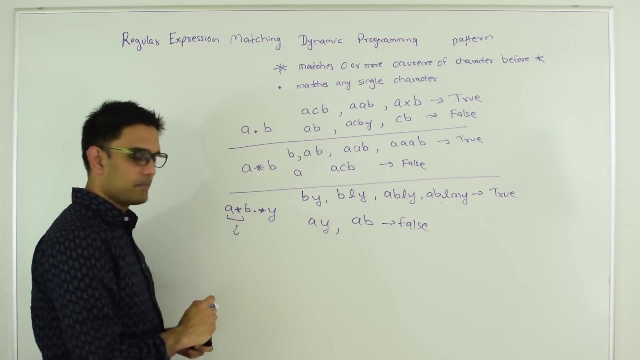 match, because there is no c in this, in this regular expression, in this pattern. Let's take one more example: a, star b, dot, star y. So here we can have zero or more occurrences of a, then we need to have one b, and then we can have zero or more. 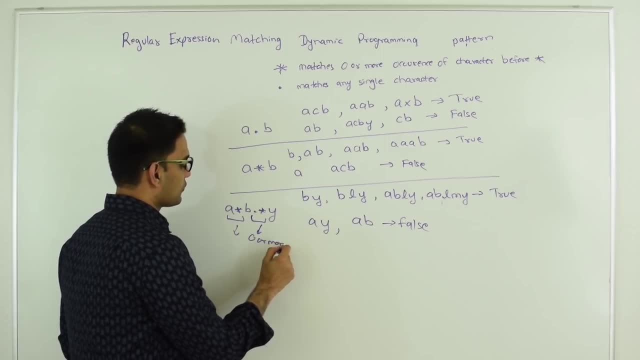 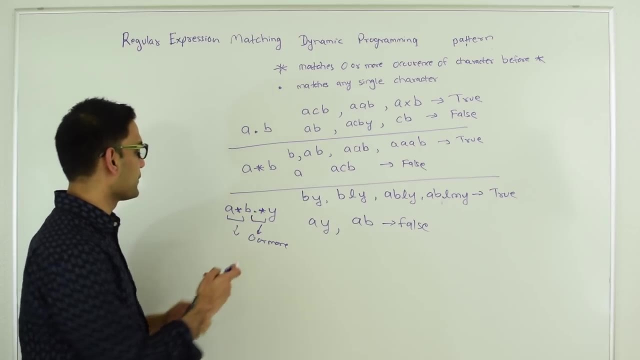 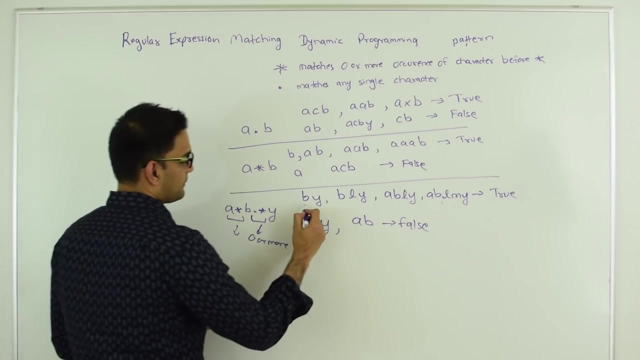 occurrences of any character. So dot star meansdot means any characterstar means zero or more number of times that characterSo between b and y we can have zero or more of any characters, and that would be a regular expression. matchSo let's see b? ySo here b? y has zero. 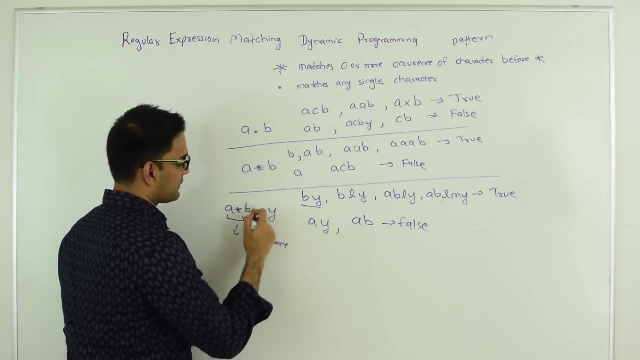 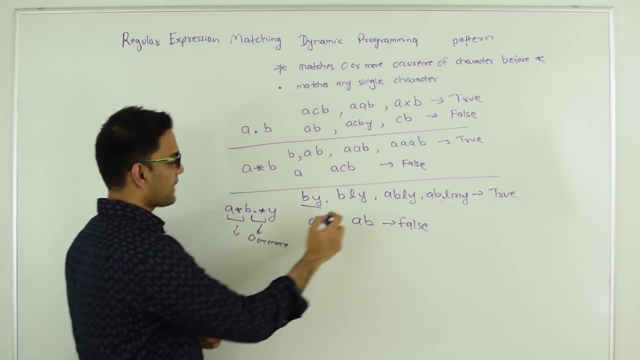 occurrences of a, then we have b and then zero occurrences of dot star, and then this is ySo this text matches this patternOn the other hand, b and y also matches this pattern, because we have one l between b and y and zero occurrence of a. 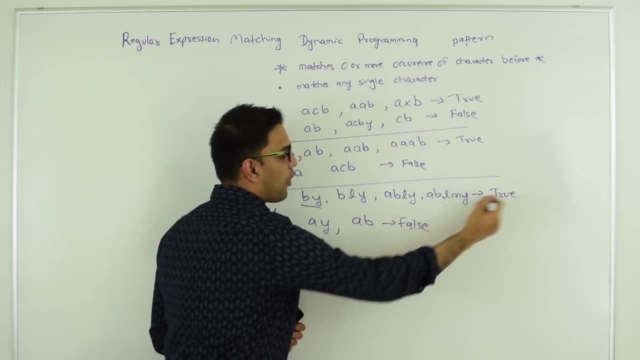 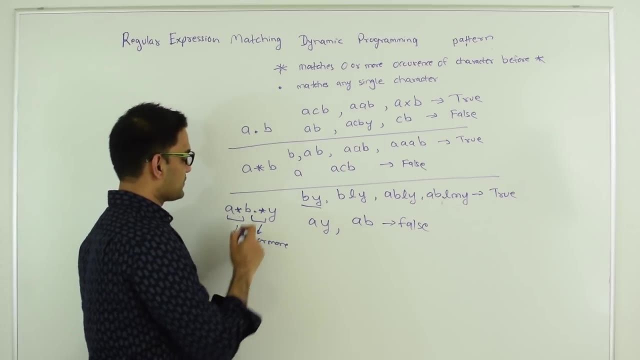 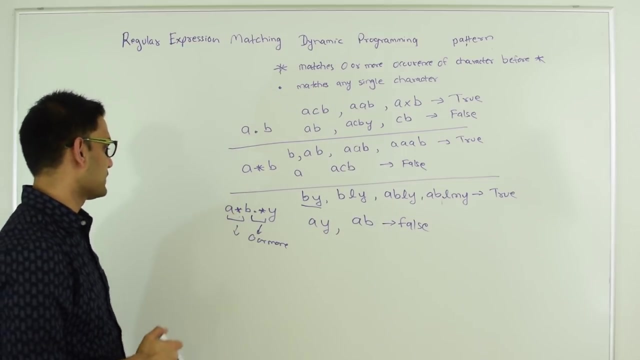 a, b, l, ya, b, l, m, yall of them are matched with this pattern. On the other hand, a- y is not a match because we need this. ba b is not a match because we need this ySo these guys arethese text doesn't matches this pattern. 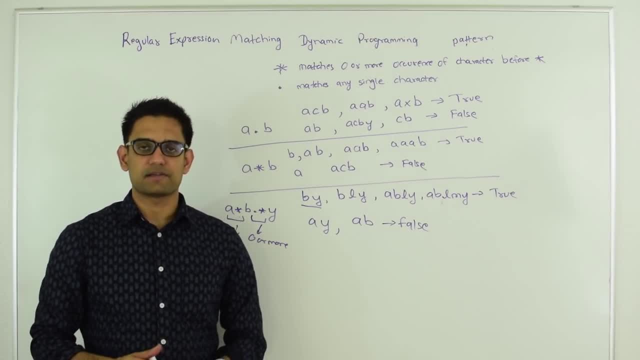 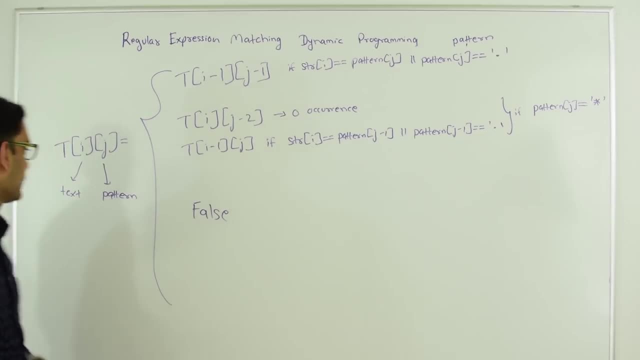 So next let's see how we are going to solve this using dynamic programSo first let's look at the recurrence relationship, or how we're going to fill up the table in bottom up dynamic programmingSo here t is a two dimensional Boolean matrix where i is the index in the text and j is index in the 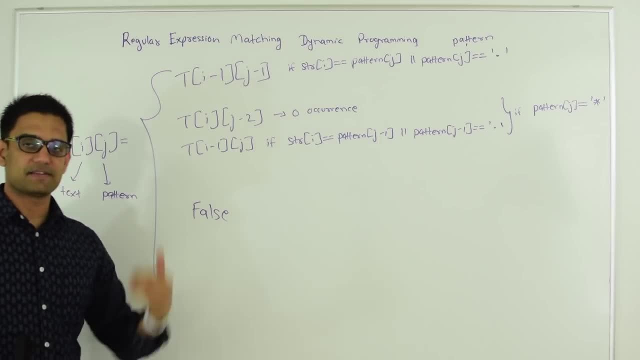 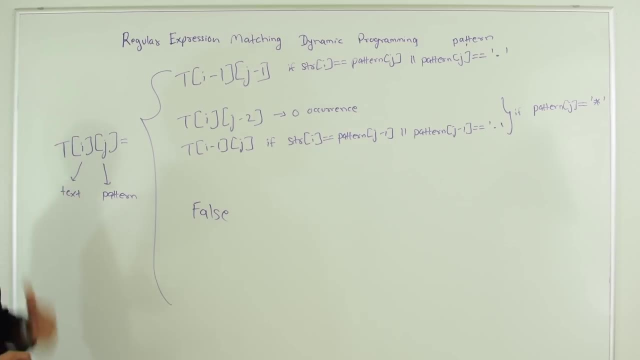 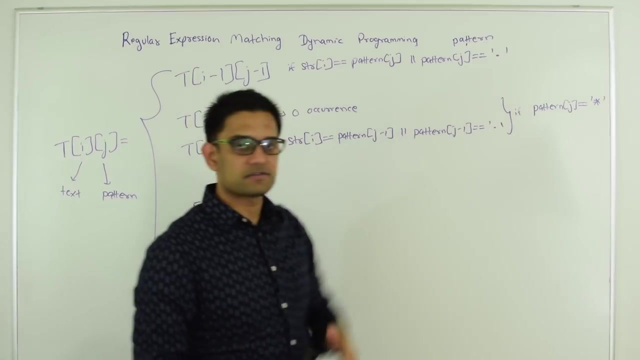 patternSo if tij is true, it means that till ith value in text and jth value in pattern, there is a regular expression matchSo how does tij gets its valueSo if string of i is same as pattern of j or if pattern of j is dot, in that case t of j? 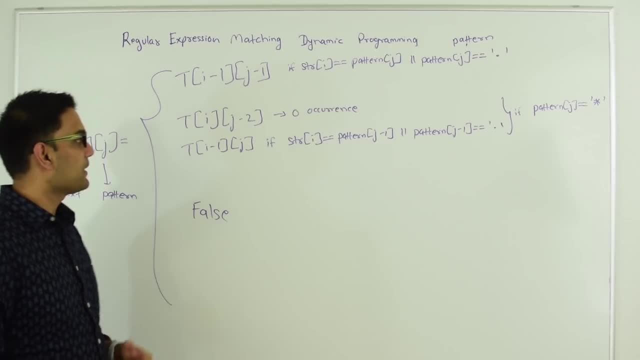 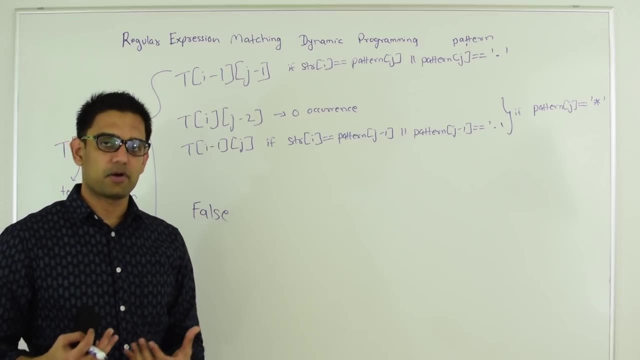 of ij will become t of i minus one. j minus oneWhyBecause value at i matches pattern at j or pattern at j is dotSo those characters are already matching. so without them or removing them from text and pattern, whatever is left, we check if that is a regular expression match. 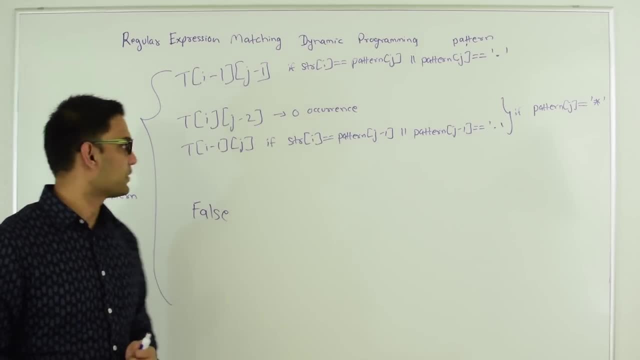 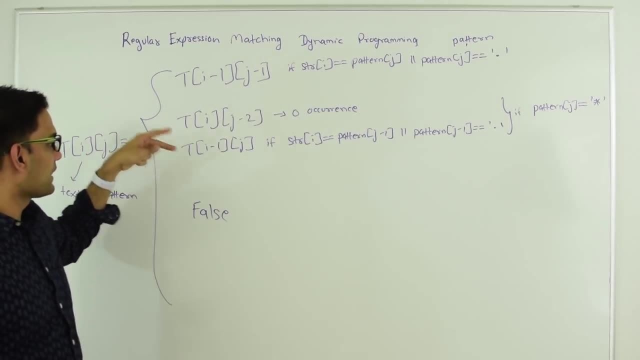 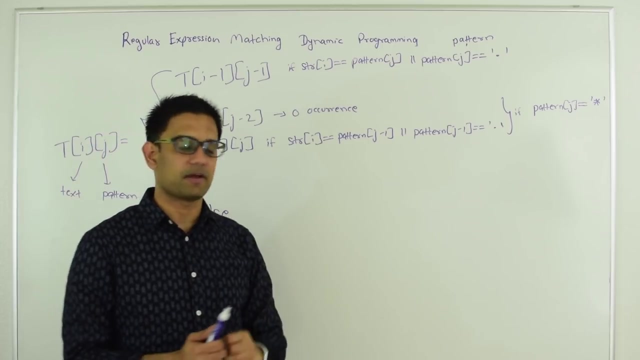 or not, and that value is coming from t of i minus one, j minus oneOn the other hand, if pattern at j is star, in that case we have two conditionsOne is we can have zero occurrences value right before this pattern, jSo at value pattern of j minus oneFor looking at zero. 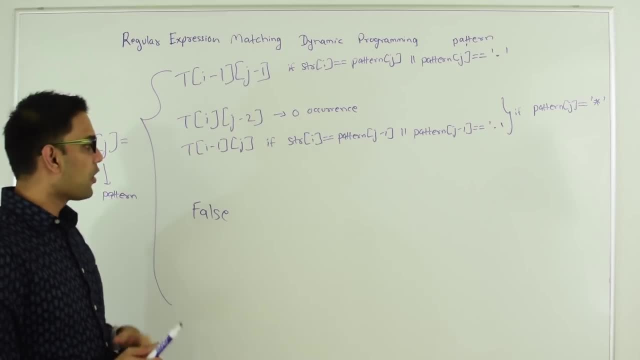 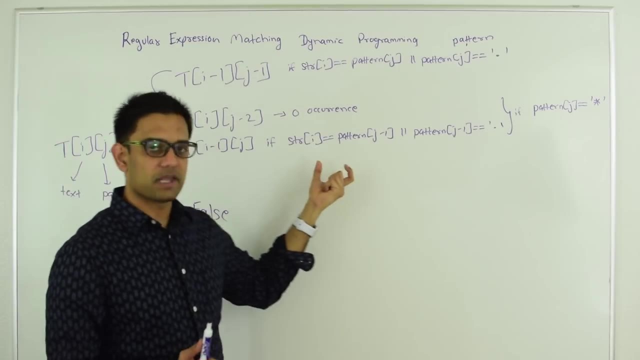 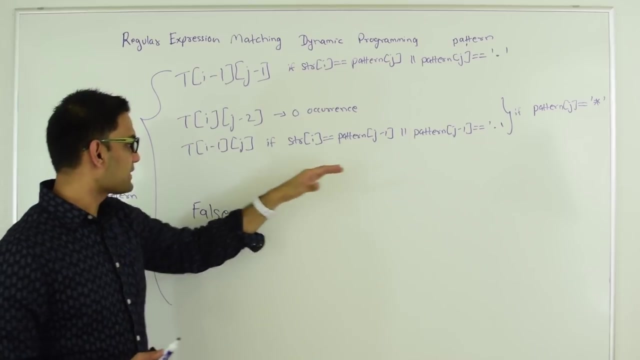 occurrence. you look at t of ij minus two or we could have one or more occurrences of the value right before pattern and we can only apply that if string at i is same as pattern of j minus one, or pattern of j minus one is dotSo in that case this takes a value of 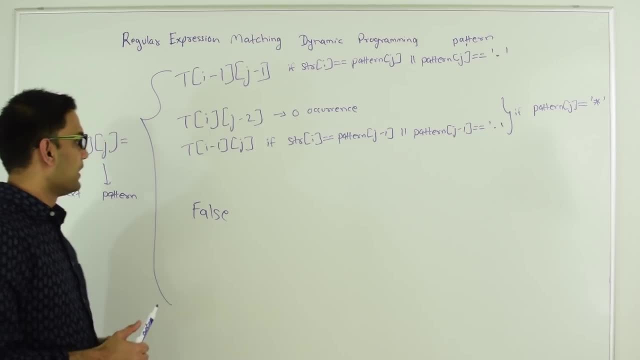 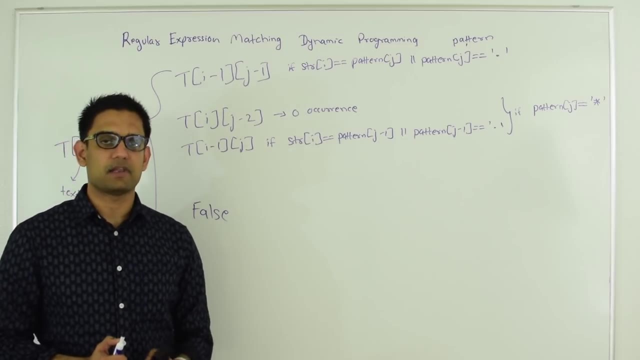 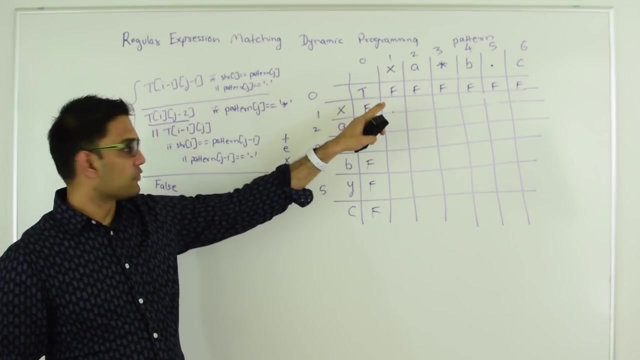 t of i minus one, jSo basically value at the top, And otherwise this takes a value falseIf this is not clear, it's ok, because I'm going to take an example and hopefully that will clarify this logic very clearlyIn this example, the pattern is going to be x, a, star, b, dot, c and text is going to be x, a, a, b, y, cSo first, 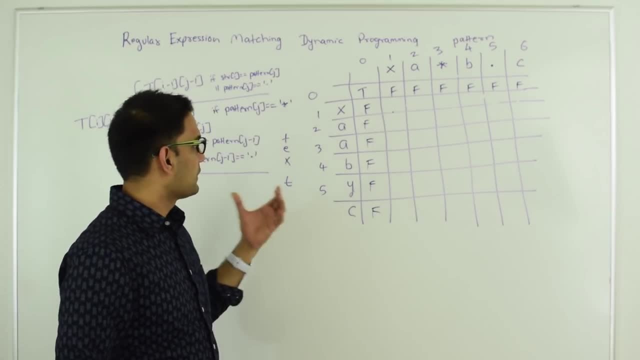 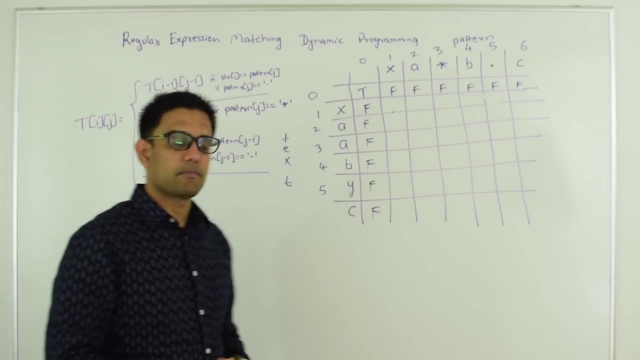 thing we do is we take a two dimensional boolean matrixThe number of rows and number of columns in this matrix is going to be one more than the left length of the text, length of the pattern. Then first thing we are going to do is we are going to initialize. 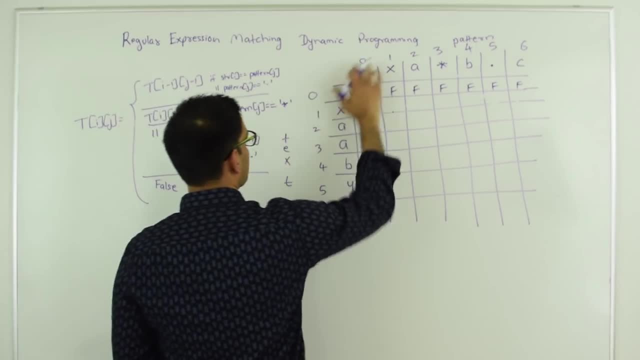 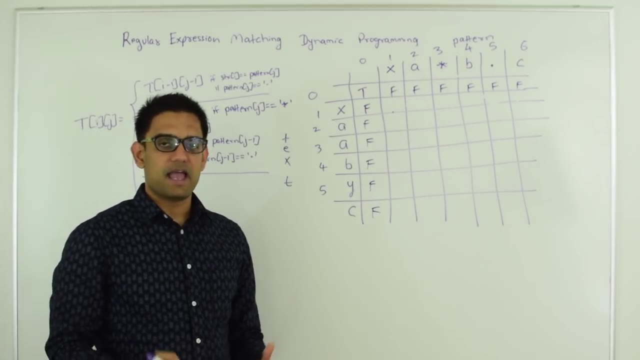 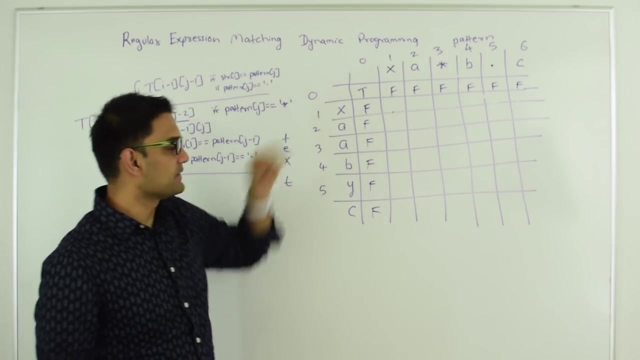 the 0th column and 0th row. So first let's look at this value t00.. So this value here I have set true. Why? Because if we have an empty string and if we have an empty pattern, then we are going to count that as a regular expression match, which is why this t00 is. 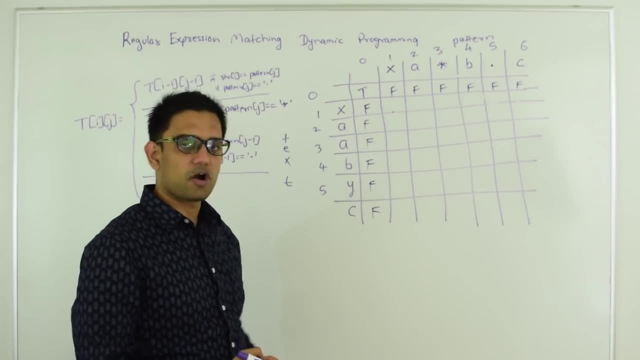 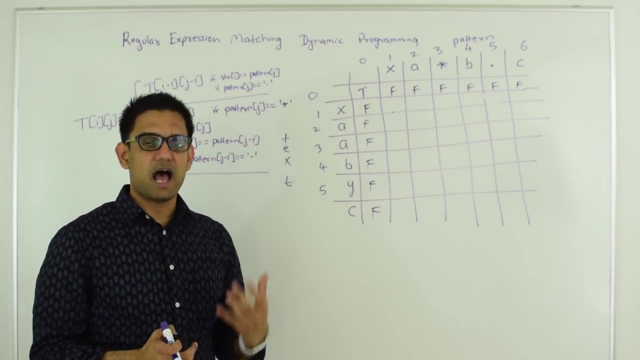 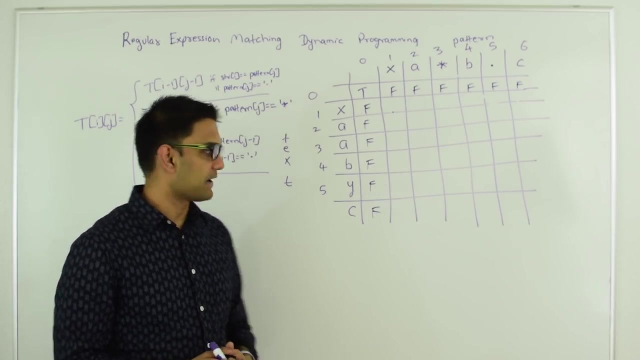 true, Then let's fill up the 0th column. So when I'm filling up the 0th column, I'm considering this: I have an empty string for a pattern and for my text I can have any value which has at least one character. If that is the case, then that will never be a regular expression. 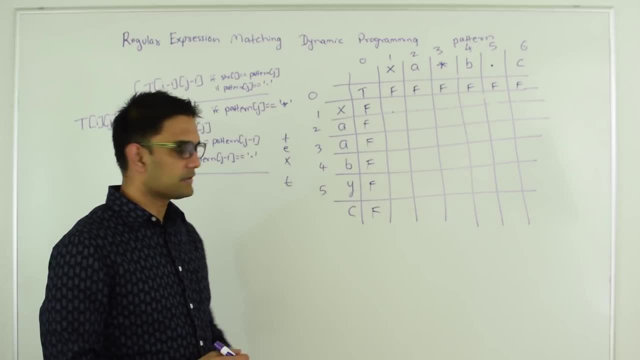 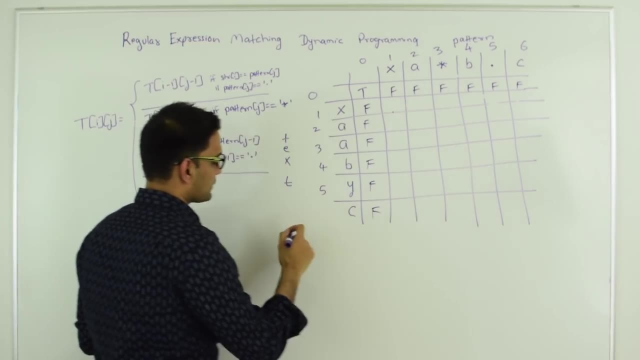 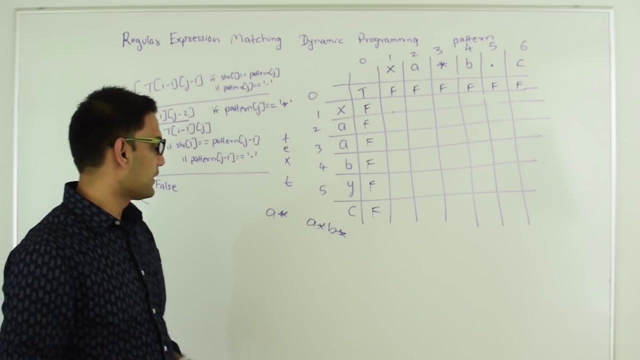 match, which is why this 0th column is all false. Now let's talk about the 0th row. So if my pattern looked something like this: A star or A star, B star, what is possible here is that this guy can match with an empty text. If a text is empty, that still has a regular. 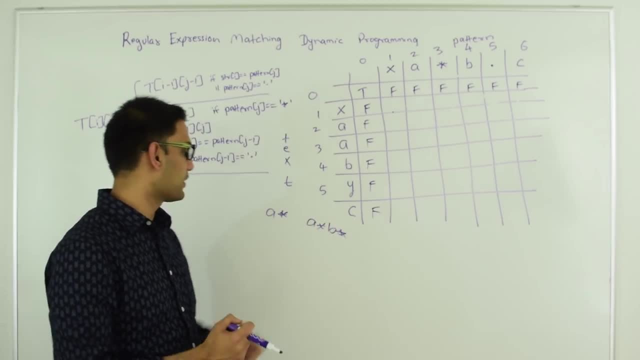 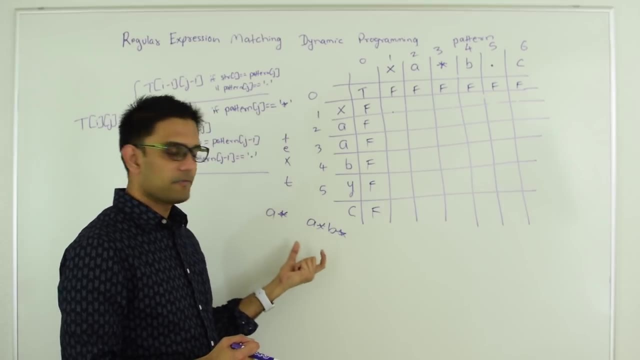 expression match with A star, B star, because we can have 0 occurrence of A and 0 occurrence of B. So if we had something like this, if your pattern looked something like this, then we would have, then we would have true values on the 0th column. 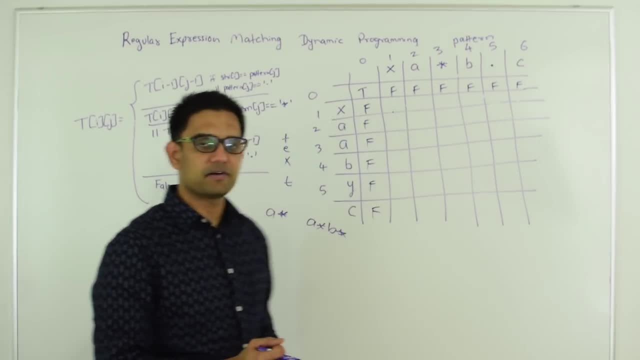 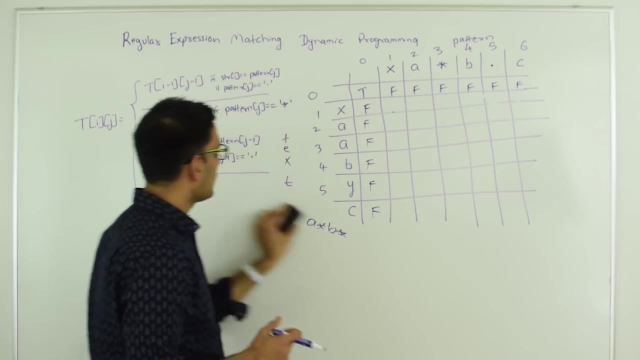 On the 0th column, 0th row, but in this case this pattern. with this pattern, there is no way that any value will be true, which is why I have set all the values as false. So now with our 0th row and 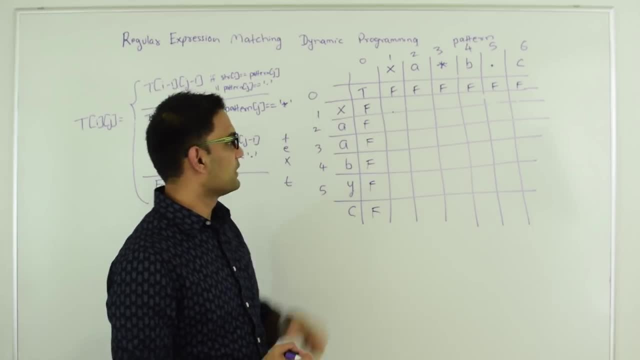 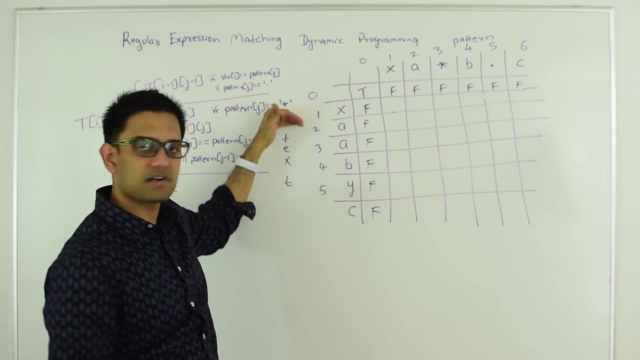 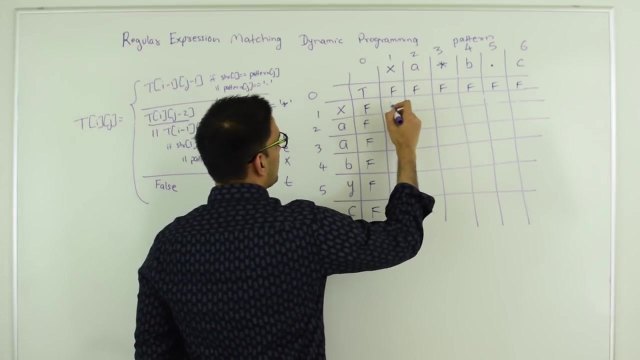 0th column set. let's move on to the t11.. For the simplicity purpose, I am assuming that my string, my text, is starting from my text index and my pattern index is starting from 1 instead of 0. So t11 and we are here. So at t11, what we are checking is: is this x same as this x? 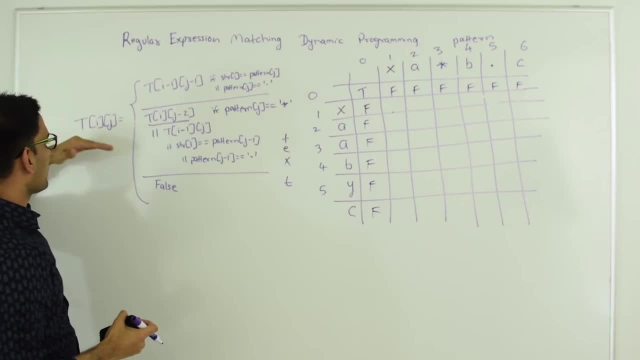 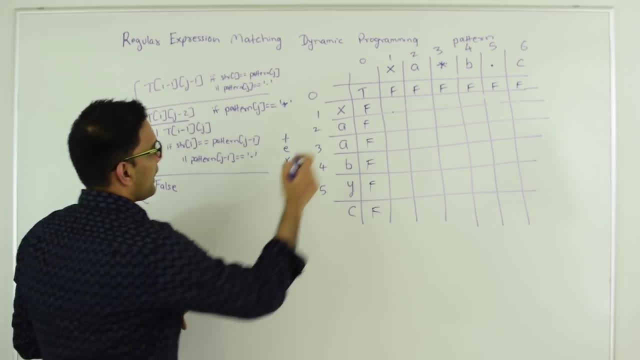 They are same. So what we are going to do is we are going to say what value tij takes. So, since string of i is same as pattern of j, t of ij becomes t of i minus 1, j minus 1.. And t of i minus 1, j minus 1. this value, diagonally, is true, so this value also becomes true. 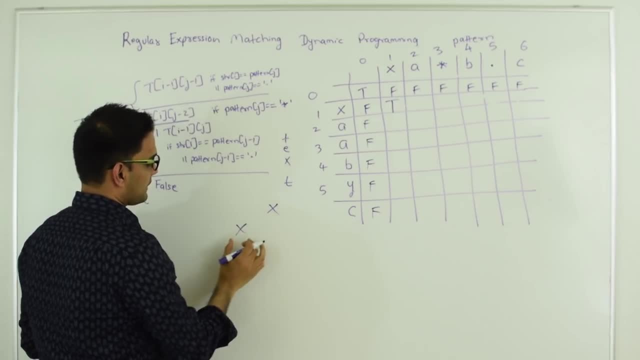 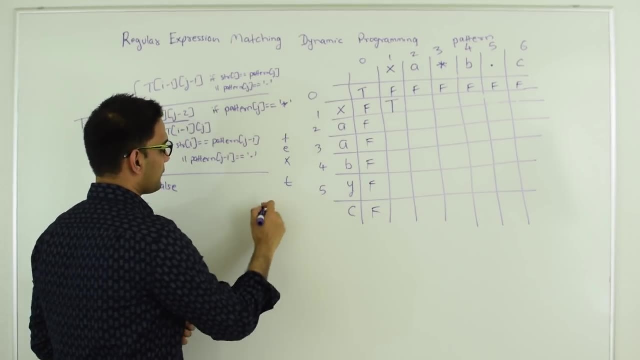 Again, if my text, if my pattern is x and my text is x, and since they are all the same, since they are a match, so we can, so we can remove them, and what we are left with is two empty strings. and those empty strings were also a match because this value is true. 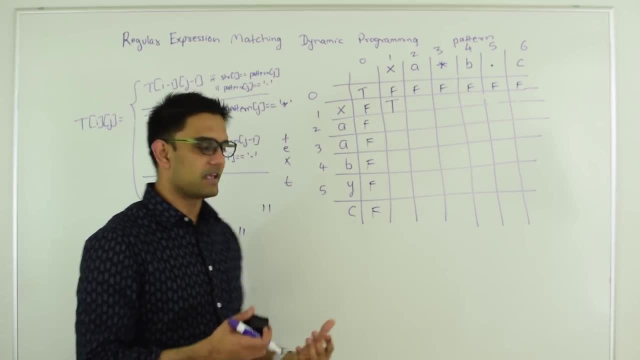 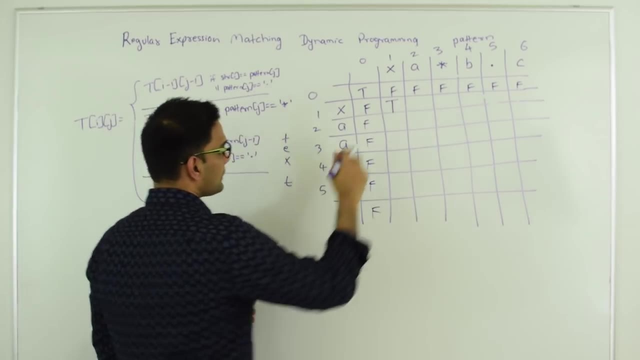 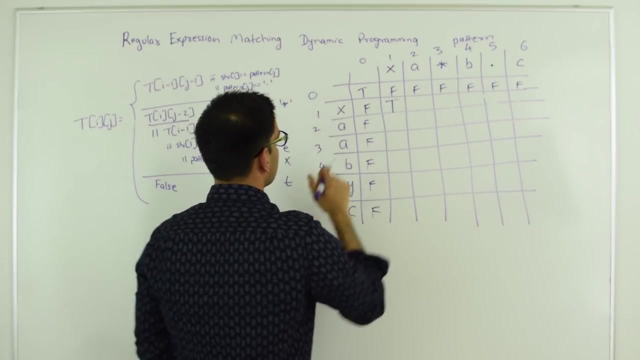 So since that is a match and adding x is same value, so adding x will also continue to be a regular expression match, which is why this value is true. Next, our we move on to the next column. Here the value the pattern is a and value of the text is x. 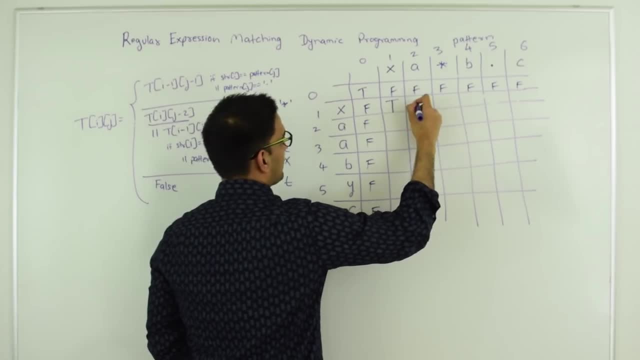 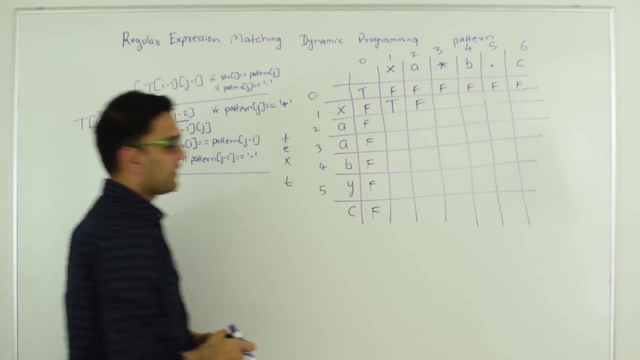 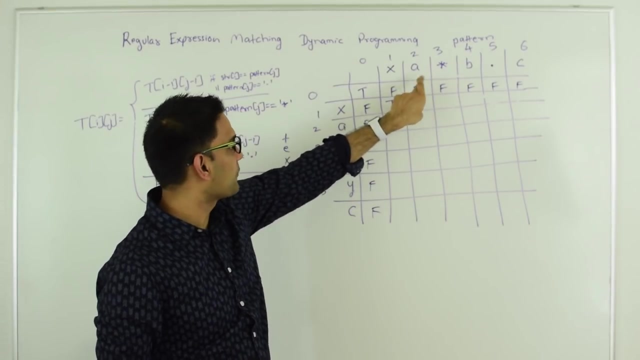 x is not same as a, so we come directly to this condition and this is false. Next, the value value of the pattern is star. So if the value of the pattern is star, we hit this middle condition. So in this case we can have zero occurrences of a character right before star, which is a. 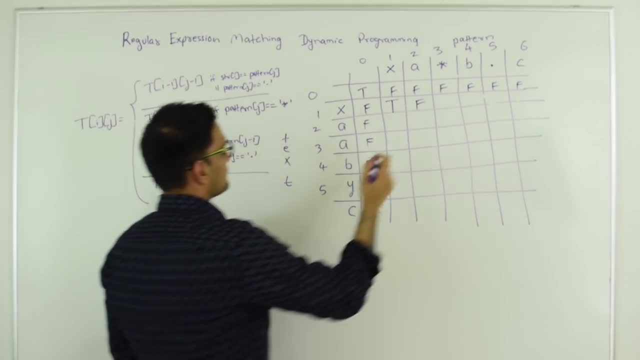 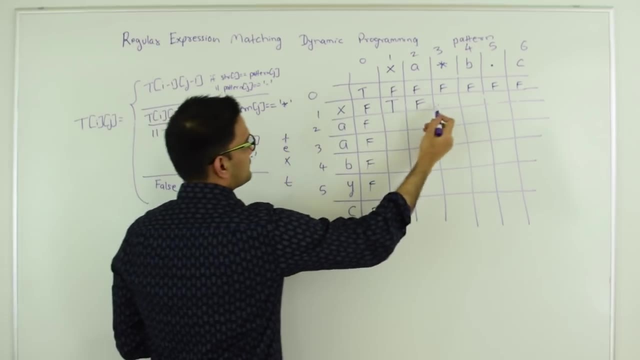 or we can have one or more occurrences of a. So in this case, for zero occurrences, what we are going to do is we are going to stay on the same row and move two back. So stay, we are on this row and we move two back and take this value. 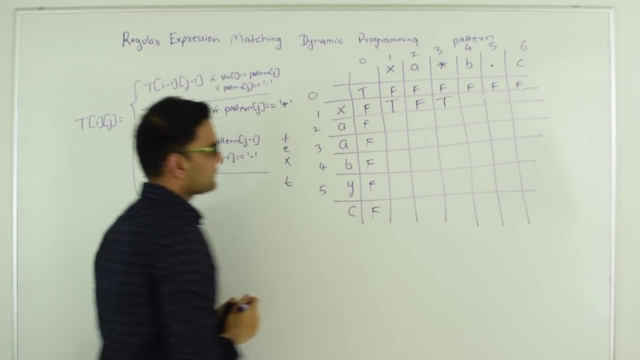 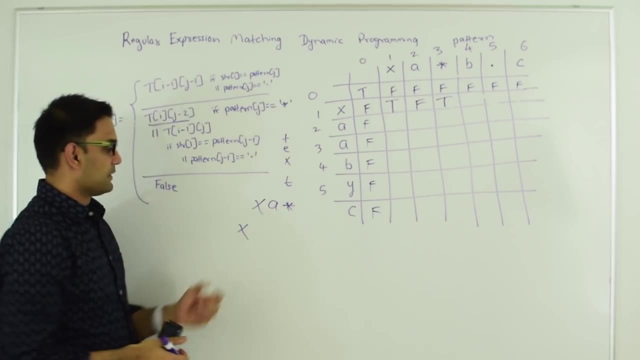 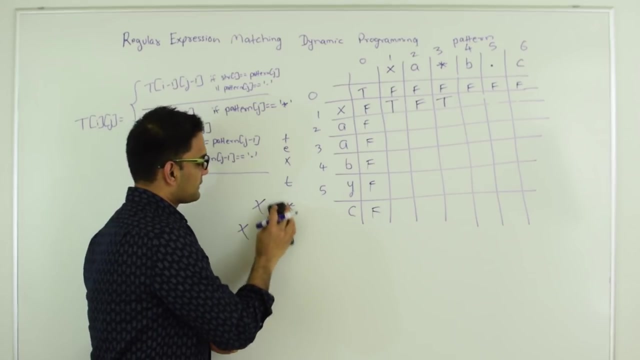 So this value is true, so we can take this value as true as well. So let me clarify. So here we have x, a star, and here we have x. Now, a star can represent zero or more occurrences. If we consider zero occurrences of a, in that case this doesn't exist and we only have x. 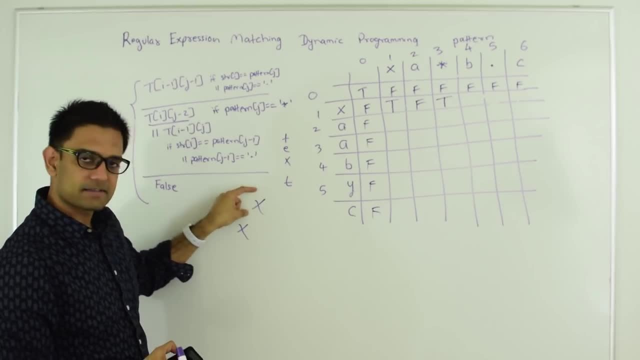 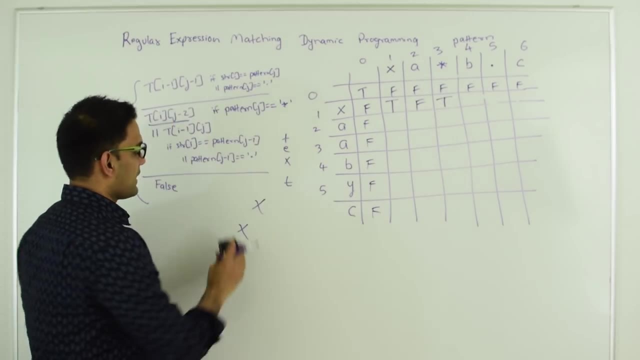 and we already know that this x matches. this x has a regular expression match with this x, because this value is true. So we can just take this value true and move it here and we can assume that there are zero occurrences of a, which is why this value here is true. 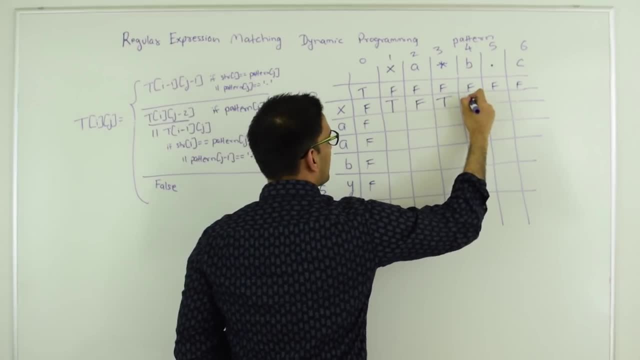 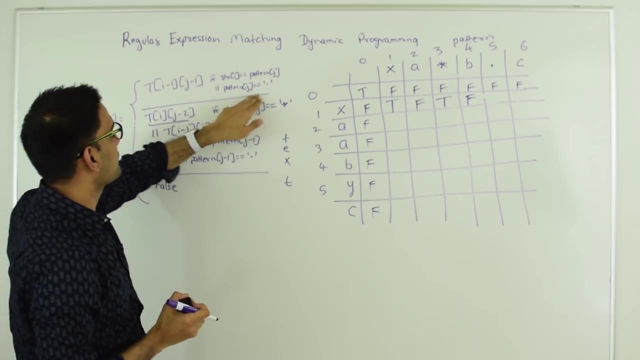 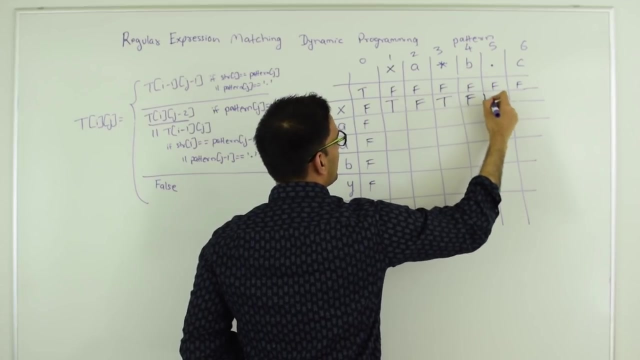 Next, b is not same as x, so this value is false. Dot is dot, matches any character. so we again hit this first condition where pattern of j is dot. So we take the value of i minus 1, j minus 1.. So the value of i minus 1, j minus 1 is false. this value here, so this value also becomes false. 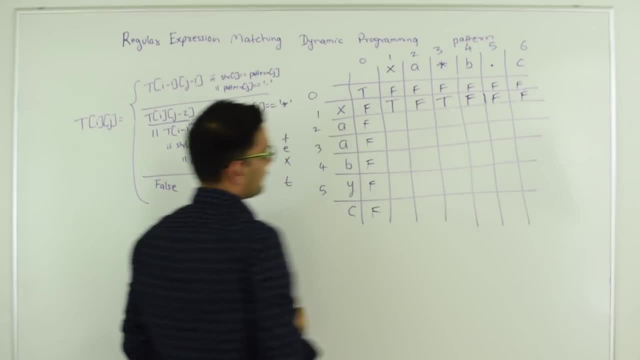 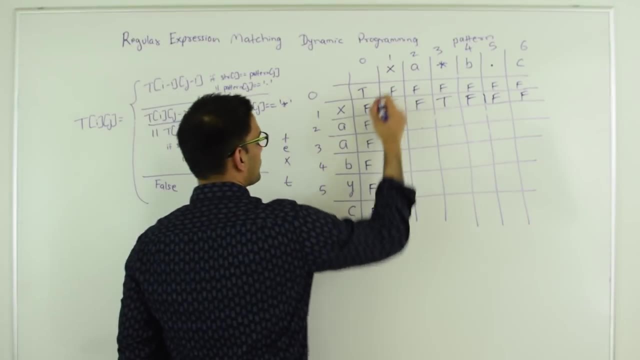 And c is not same as x, so this value becomes false. Next, let's fill up the next row. So now we are going to match this a and this x, So the values are different. so we take this false value and this becomes false. 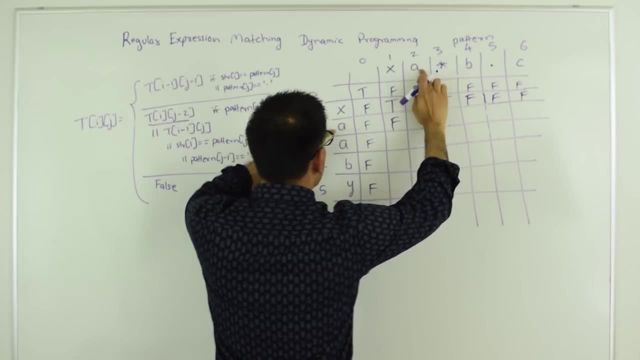 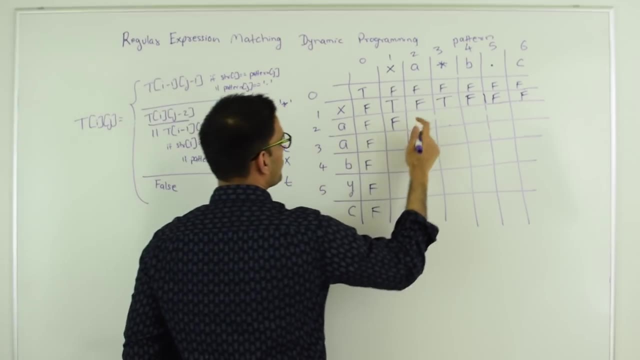 Then we match this a and this a, So this a is same as this a. so we hit this first condition and take the value of t of i minus 1, j minus 1.. So this value true here, So this value also becomes true. 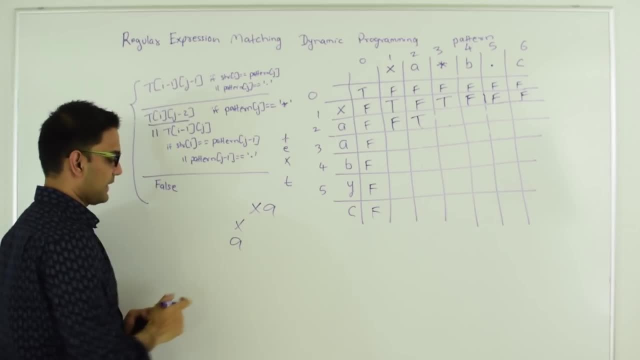 Let me clarify. So here, our pattern is xa, our text is xa. Since this a matches this a, then we are just going to check without them: is rest of the, is rest of the regular pattern, matches with the text or not? and it does, because this value is true. 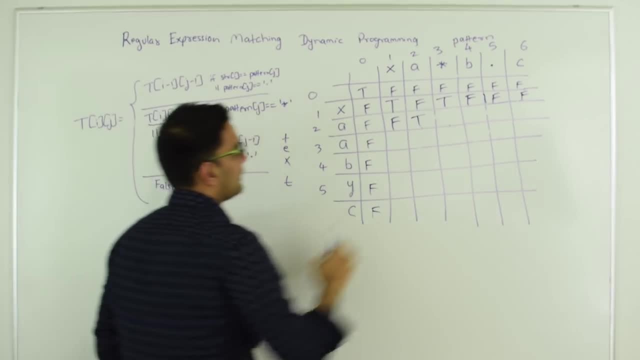 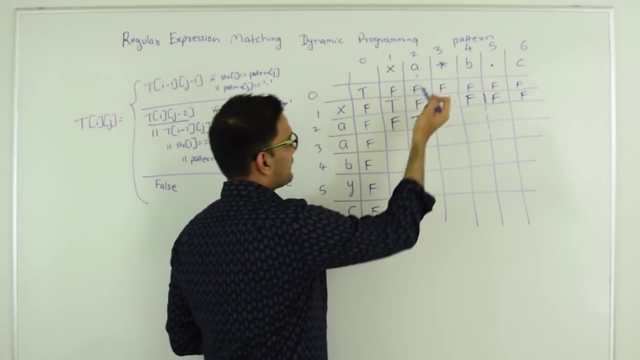 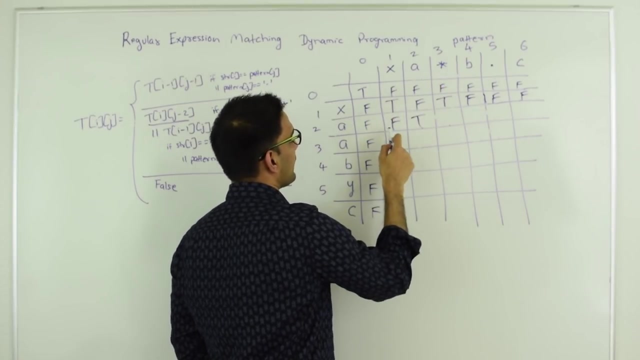 So we just take that value here. So the next character after this is star. So if it's a star we hit this middle condition. So first we check: is does counting zero occurrences of a work? So if, to look at that, we go two steps back and this value is false, 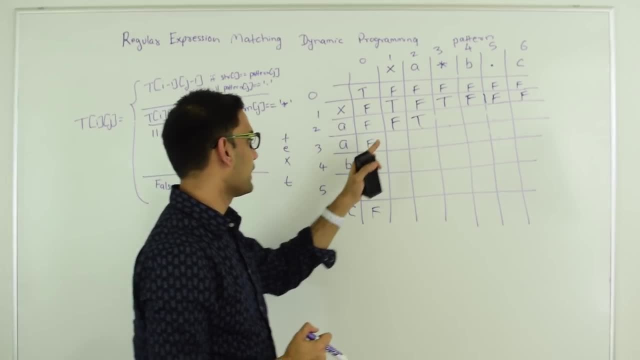 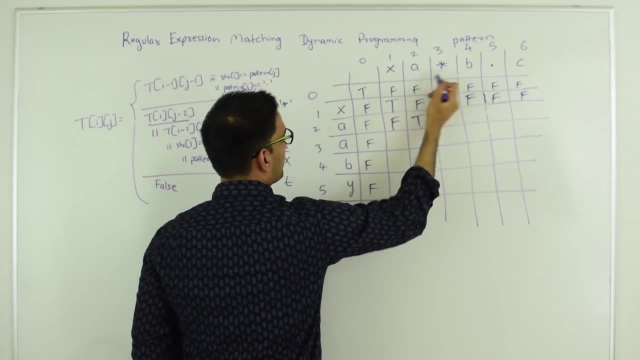 So, since this value is false, it means that we cannot consider zero occurrences of a. So then, we are going to check: is the character before star, is that same as this character? The character before star is a which is same as this character, which is this condition here. 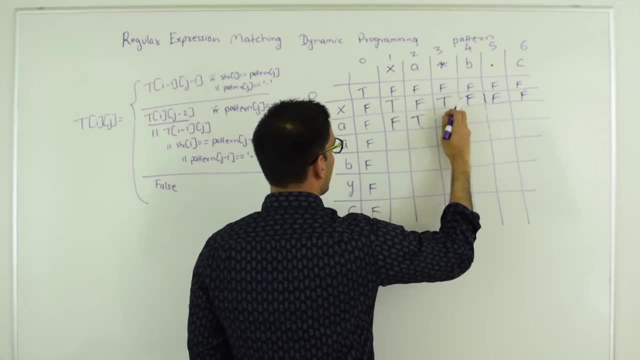 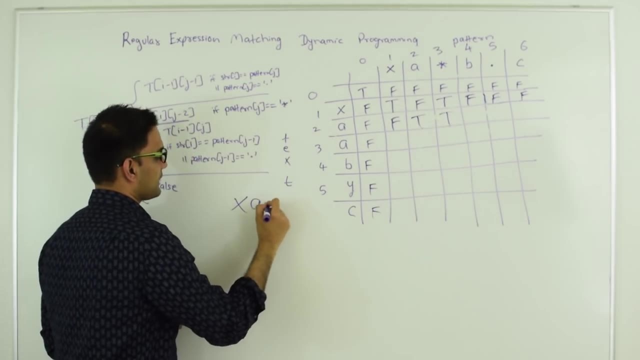 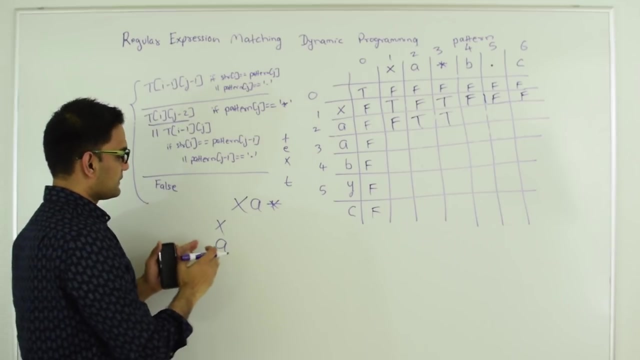 So then what we can do is we can look at the value at the top And this value is true, so this value becomes true. So let me clarify: So we have xa star and we have xa. So first we try to see that does zero occurrence of a works. 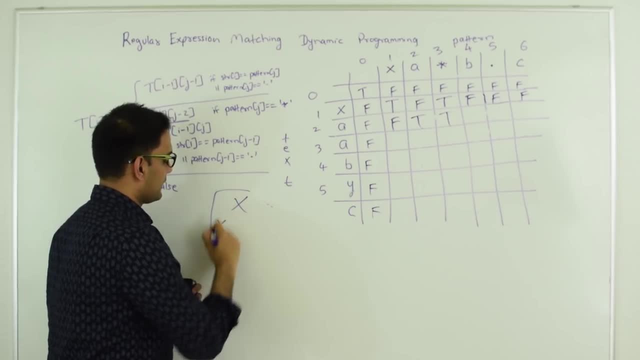 For that we get rid of a star and we see that is this a regular expression match? And for that we check here. and that is not a regular expression match. If the pattern is x and if my text is xa, it's not a regular expression match. 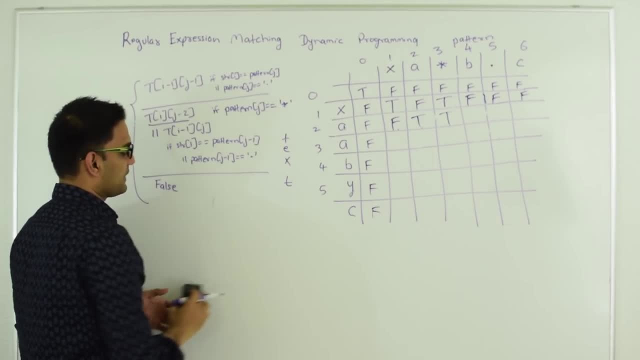 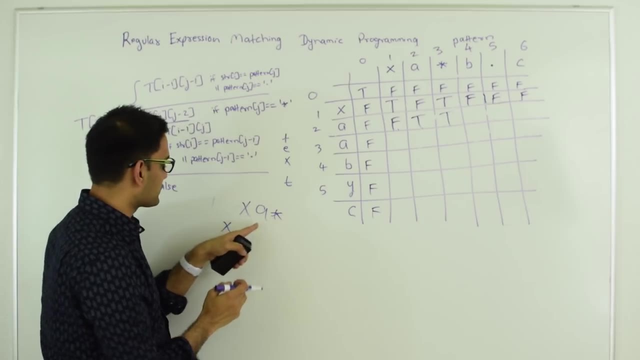 So that value is false. So then we check. can we consider one or more occurrences of a. So, since this character, the character right before star, was a which matches with this a, So then we can consider this as a part of this a star. 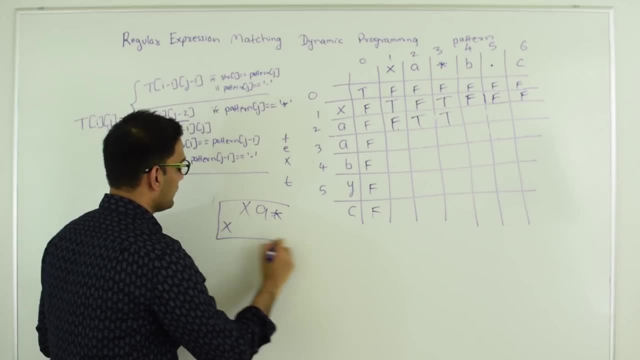 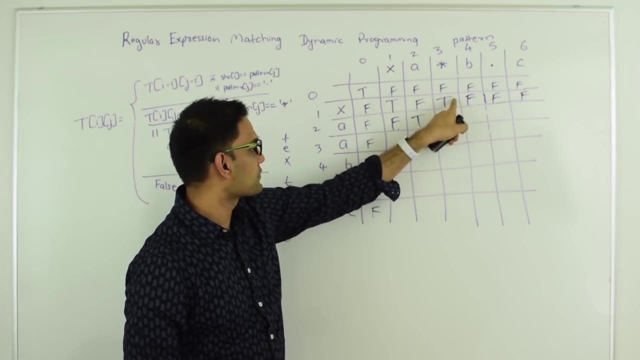 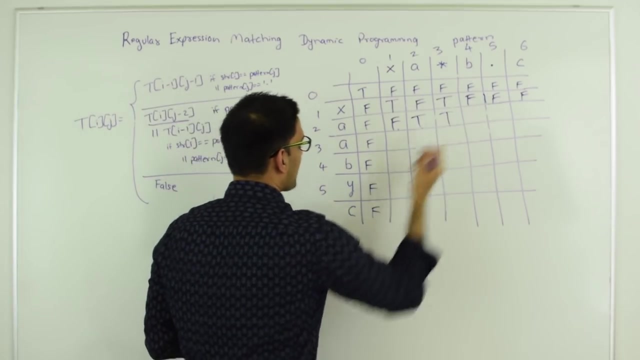 So we can get rid of this a and we check: is xa star a regular expression match with x? And that value is stored right here- the value at the top of the square we were filling- And xa star is a regular expression match with x, which is why we took that value as t. 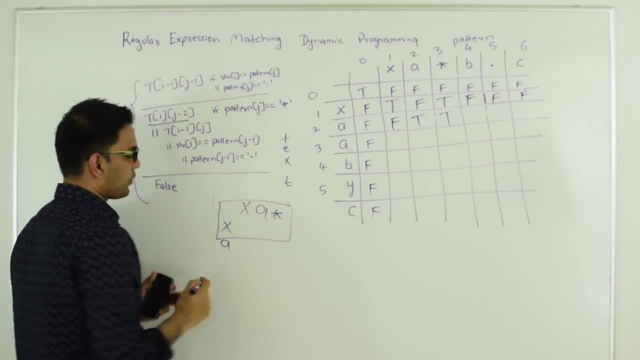 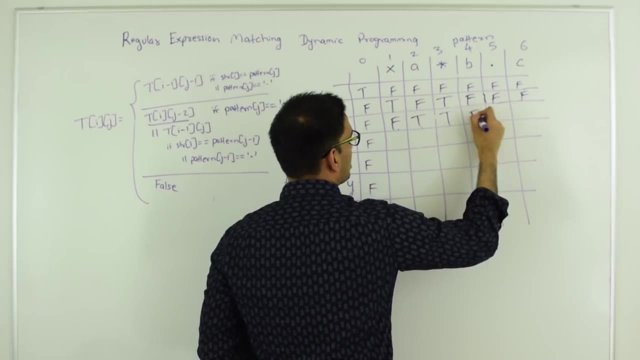 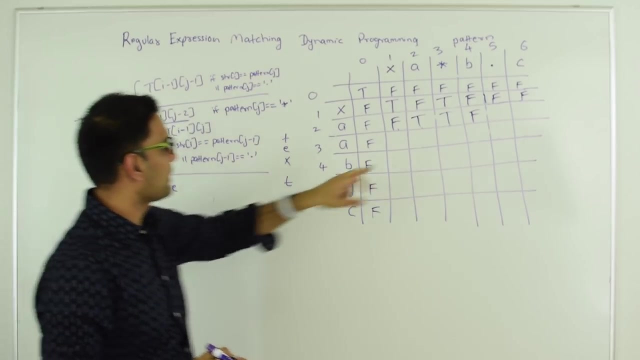 So basically adding a is also going to be a regular expression match. Then a is not same as b, so this value is false. Dot can be any character. So we hit this first condition and look at t of i minus 1, j minus 1.. 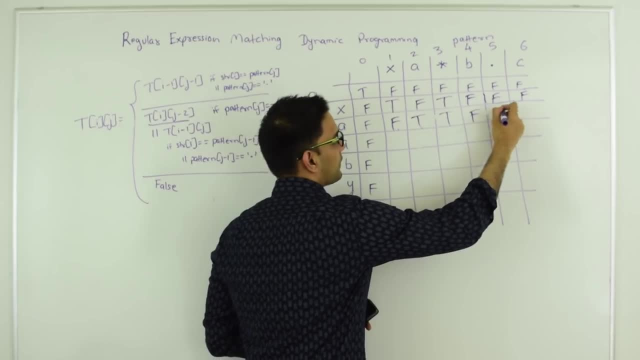 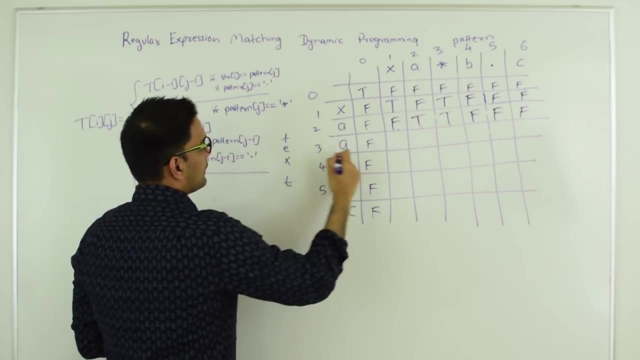 So we look at the diagonal value and that is false. so this becomes false. And c is not same as a, so this value is also false. Let's move on to the next row. So a is not same as x, So this value is false. 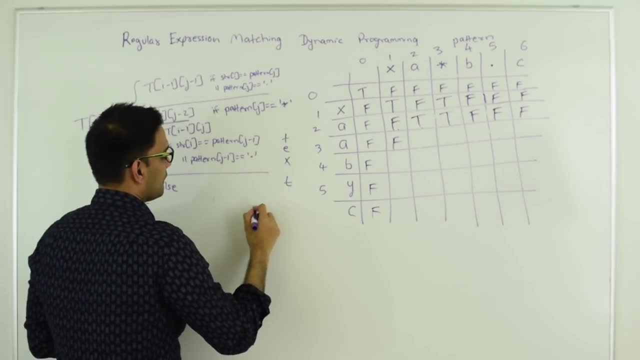 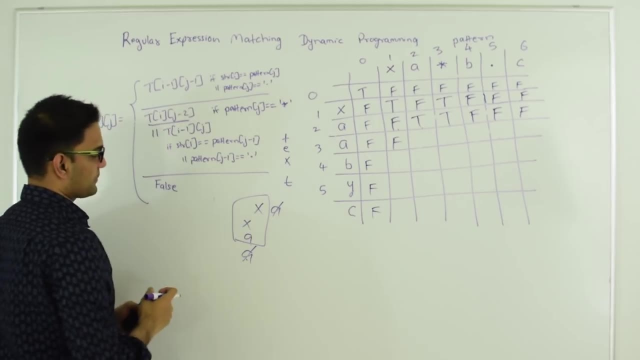 a is same as a. so we look at the diagonal value, So we have xa and we have xaa. So this a is same as this a. so we check: is rest a regular expression match? So this value is not a regular expression match, so this value also becomes false. 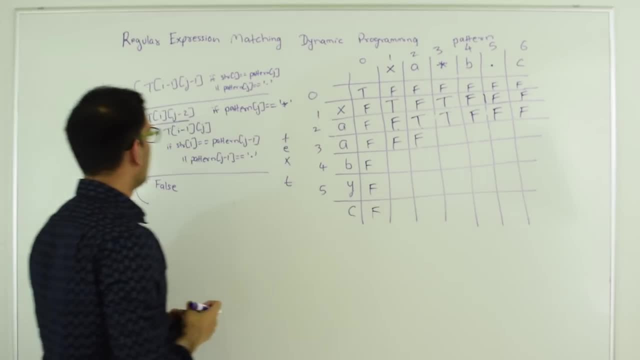 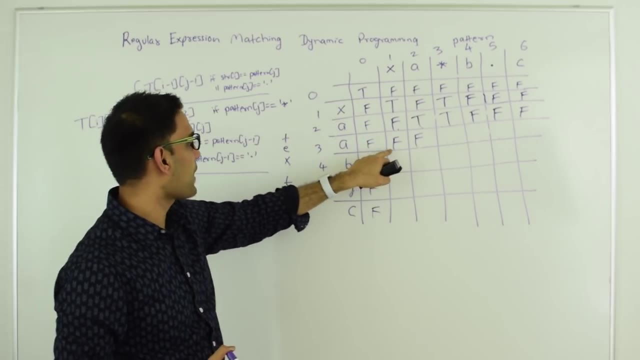 So now our next character in the pattern is star, So we hit this middle condition. So first we check: does skipping? does having 0 occurrence of a work To do that, we go 2 steps back and this value is false. So having 0 occurrence doesn't help. 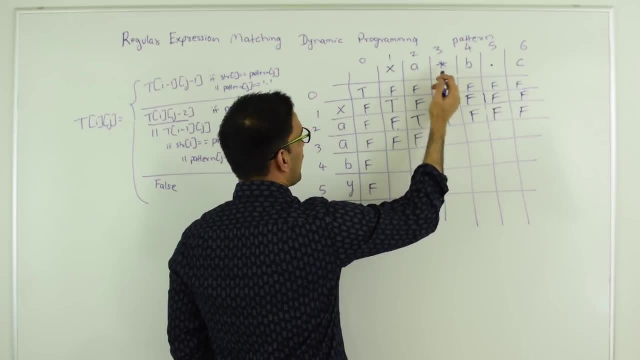 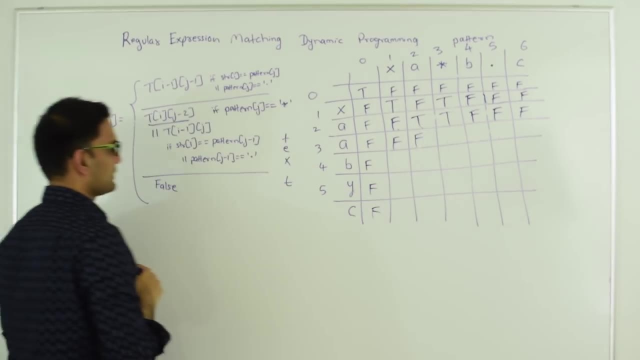 Then we check: is the character before star same as this one? So this is a and this value is also a. So then we can look at the value at the top. So the value at the top here is t. So the value at the top is true. so that's why this value will also become true. 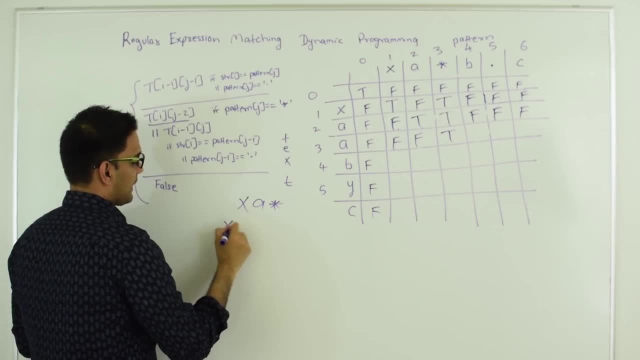 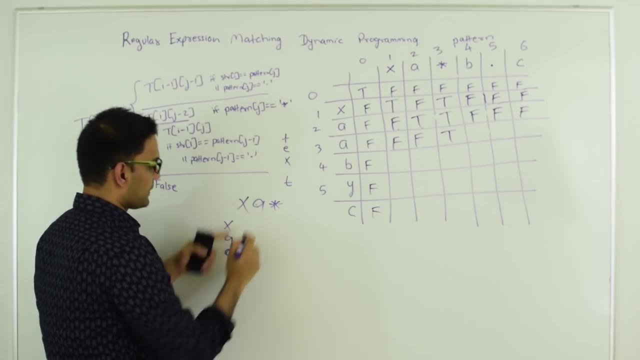 Again, let me clarify: xa star, xaa. So since the character right before this star is a, So this a could be the part of this a star. So we don't consider this a at all And c is rest of this, a regular expression match. 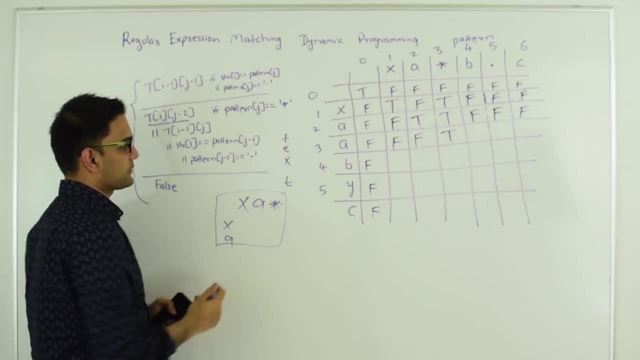 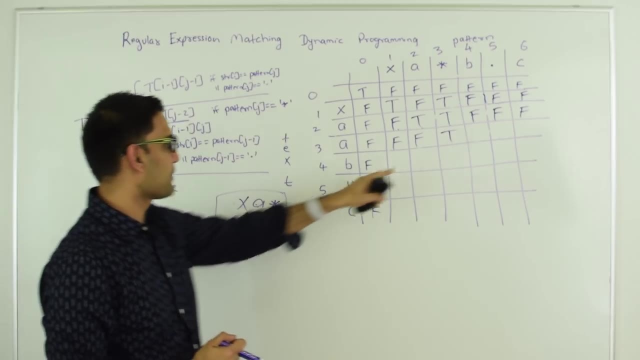 And that value is stored right here, And this was a regular expression match, So we can use that value to infer that adding a is also going to continue to be a regular expression match, Which is why this value is true And which is why we look one row up. 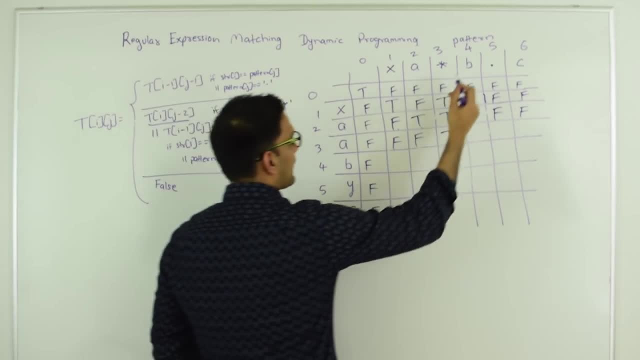 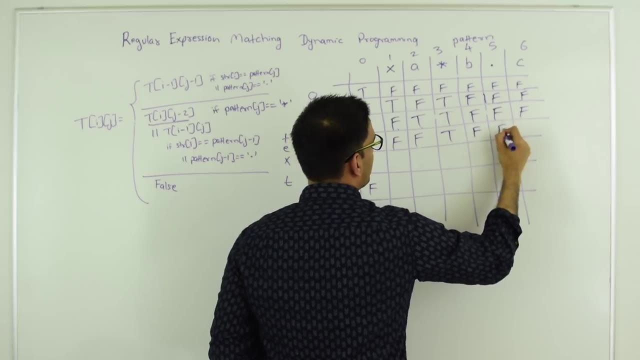 t. Next, b is not same as a, So this value is false. Dot matches with any character, So we look diagonally: This value is false, So this becomes false And this will be false. Finally, we hit b, So b is not same as x. 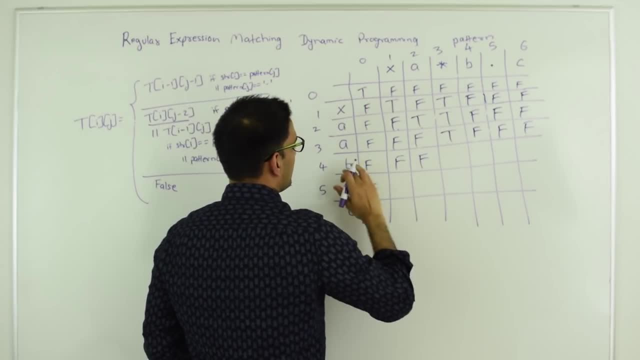 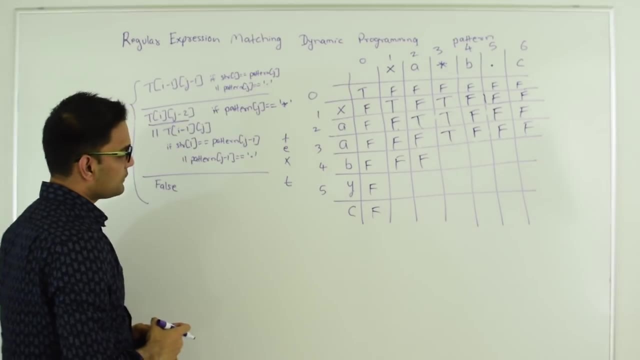 So this value is false. b is not same as a, So this value is false. We hit star, So first we check: is zero occurrence of a. So for that we move two steps back. This value is false, So zero occurrence of a doesn't work. 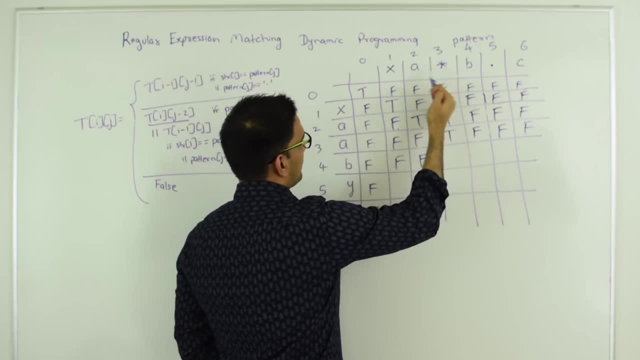 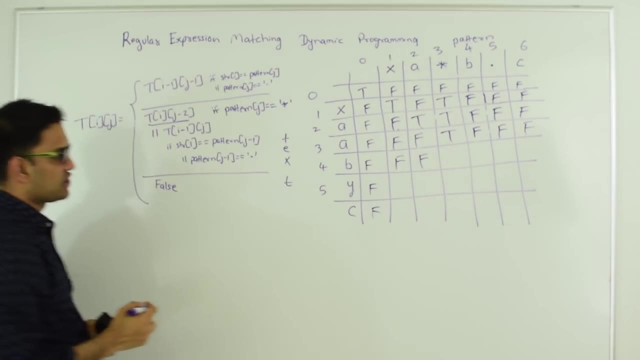 Then we are going to check: is the character right before star same? So character right before star is a And that a is not same as b. So we cannot even apply the other condition, t. So this is false. This b is same as this b. 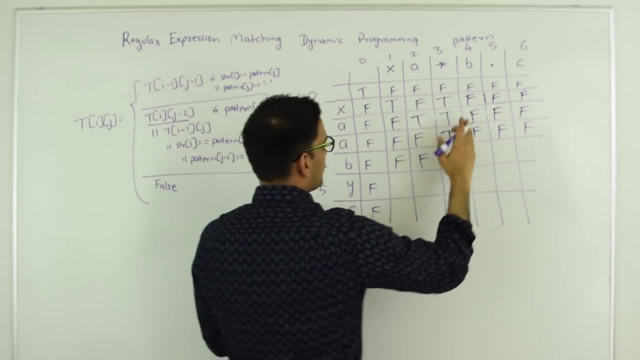 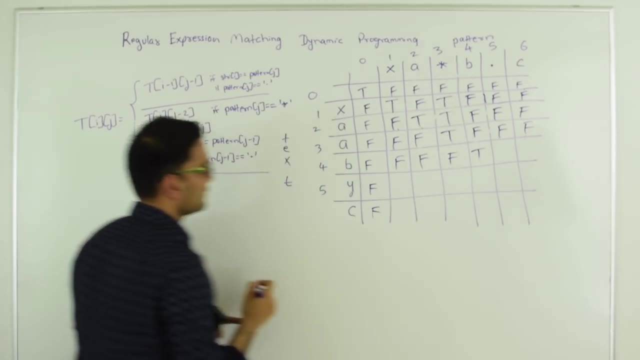 So then we are going to check. We hit this first condition And we are going to check. without these two b's is rest of the regular expression a match, And that value is stored right here And that is a match, So this is also a match. 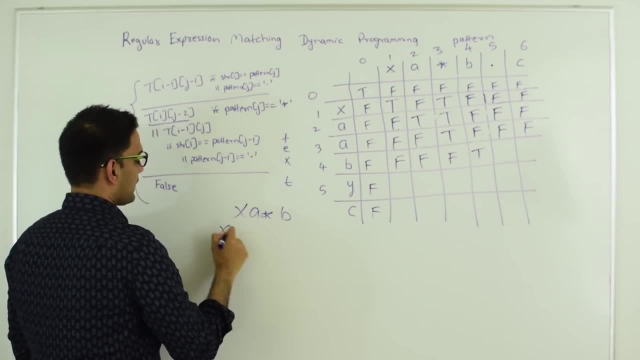 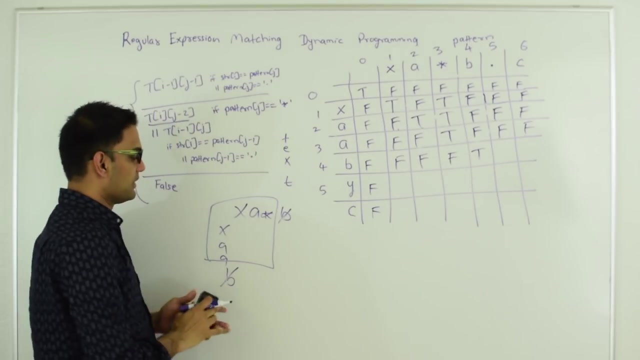 Again, x a, star b and x a, a, b, So this b and this b matches. So we get rid of them and see, is rest of the regular expression a match And that value is coming from here And that was a match. So we just reuse that value to derive that adding b will continue to make them a regular expression match. 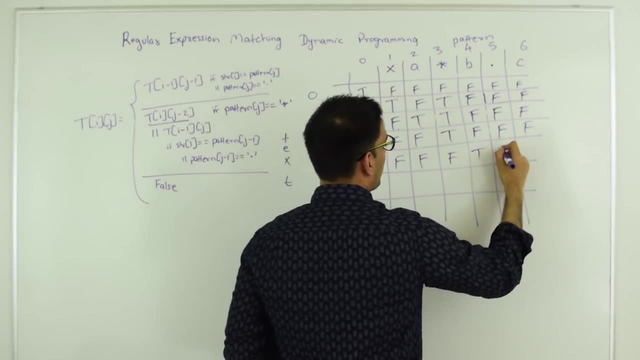 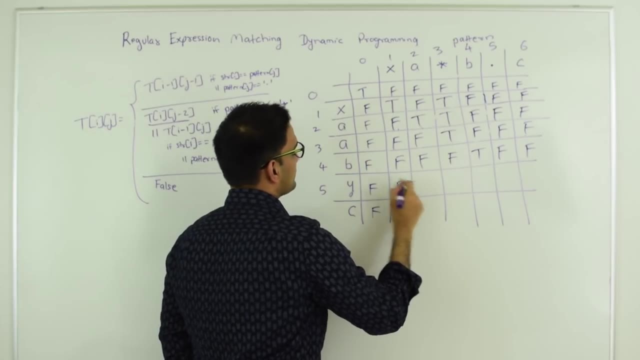 b dot can take any character. So we look diagonally up, This value is false, So this is false And this will be false. Now our character is y. y is not same as x. False y is not same as a. 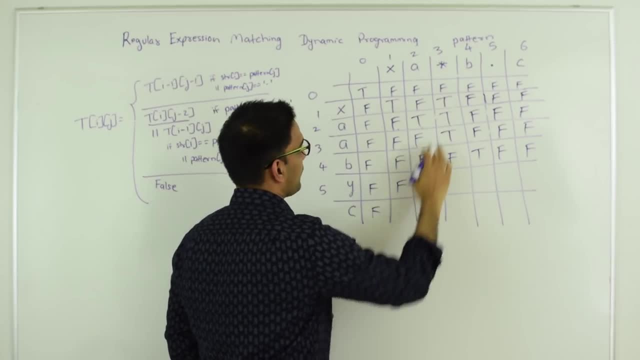 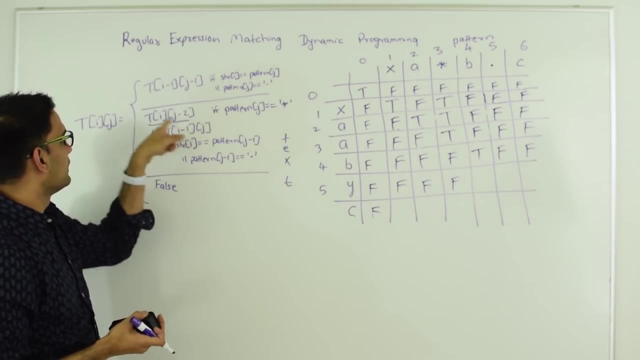 False Star. So we look two back. This is false And character right before star a is not same as y, So this will be false. So none of these two conditions, This condition and this condition, doesn't work. y is not same as this. 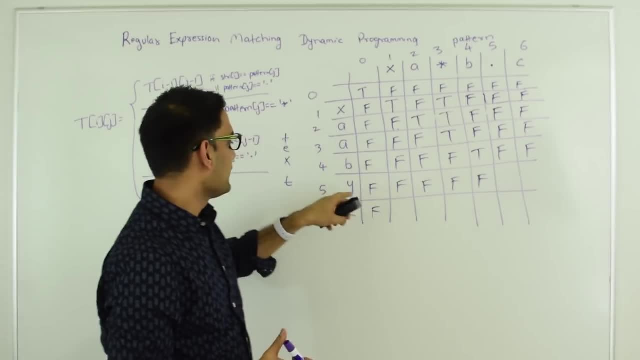 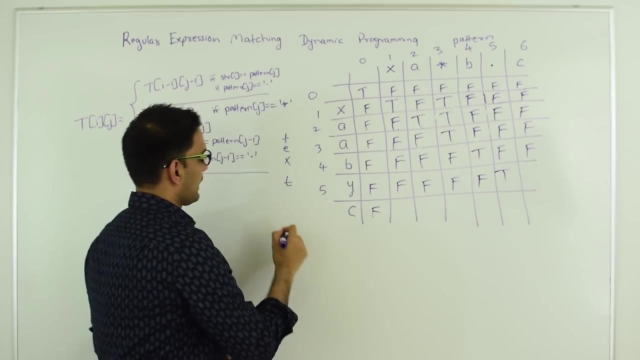 So this is false. Dot can take any character, So dot can take y. So then we look at the diagonal value. Diagonal value is true, So this becomes true Again. we have x, a star, b, dot, c, x a, a, b, y. 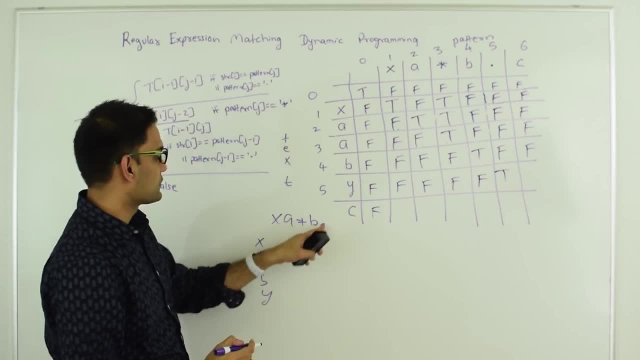 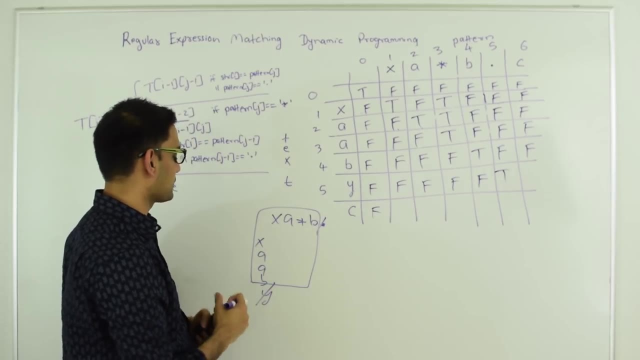 So b dot, So this dot can match with y, So we get rid of them. And c is rest of the string and text and pattern, a regular expression match. They are Because this value is true, So this value also becomes true. 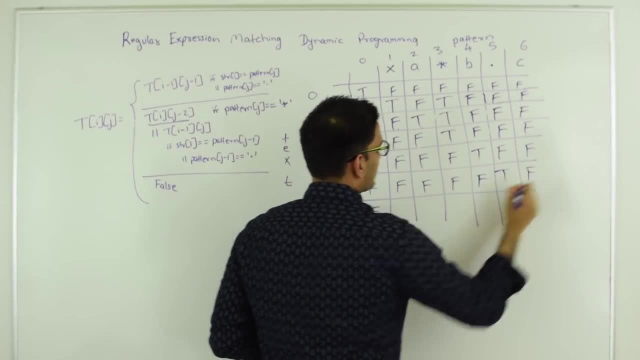 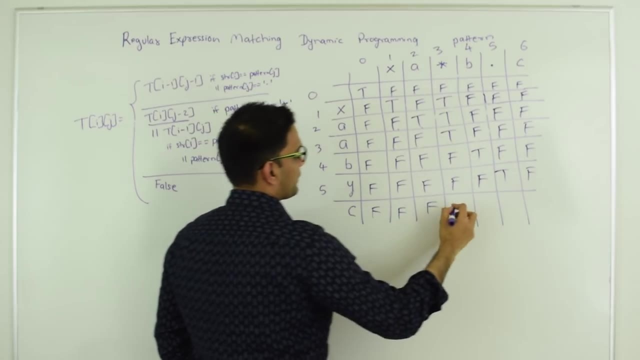 And finally, y and c is not a match, So false. And c and x is not same, So false. False Star will not work with c, So false. False Dot and this guy is same, So we look diagonally. 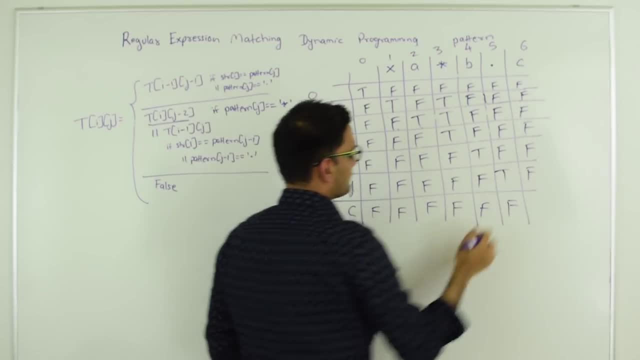 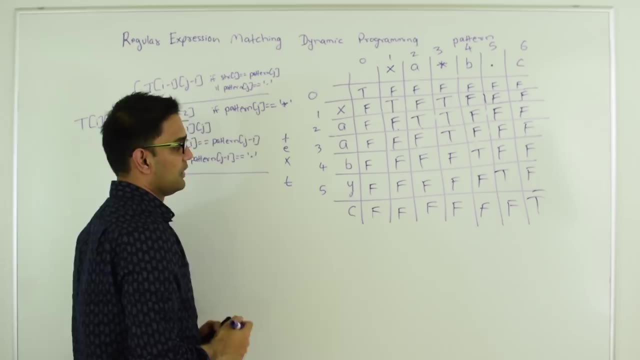 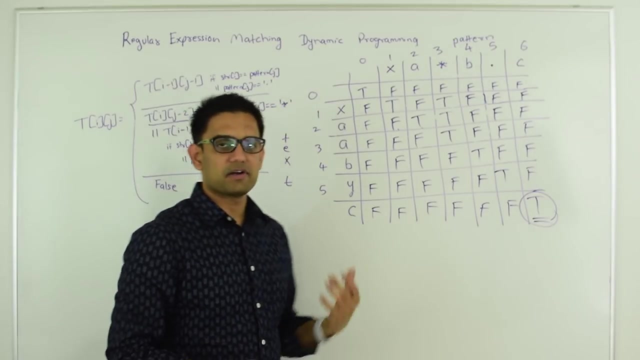 This value is false. And finally, this c is same as this c. So again we hit this first condition and we look at the diagonal value And that value is true, So this also becomes true. So this is our final answer. So this pattern and this text do have a regular expression match. 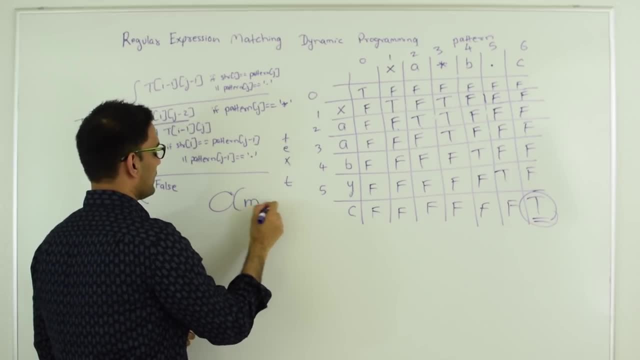 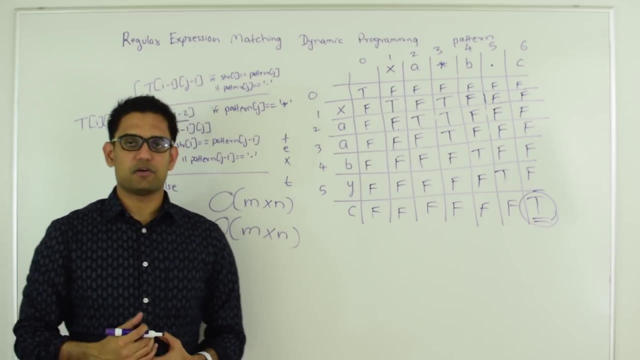 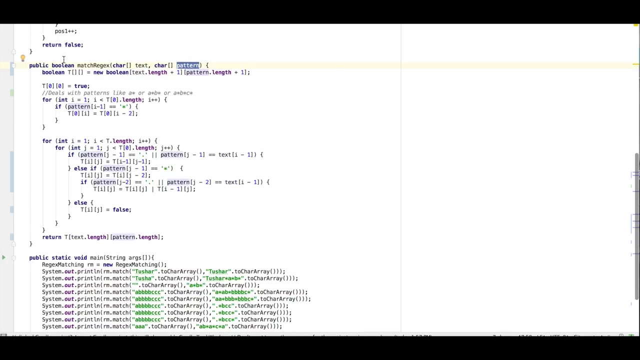 So the time complexity for this algorithm is o of m into n And space complexity is also o of m into n. Next let's look at the code for this algorithm. The main function here is match regex. It takes in a character array text and a character array pattern and it returns boolean saying: 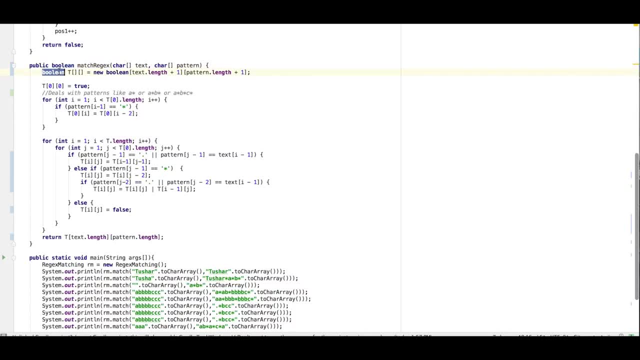 that this pattern matches the text or not. First we initialize a two dimensional boolean array, t, where the number of rows is text dot length plus one and number of columns is pattern dot length plus one. Then, as we discussed before, t is true. This for loop here deals with the zeroth row, where we set some values in the zeroth. 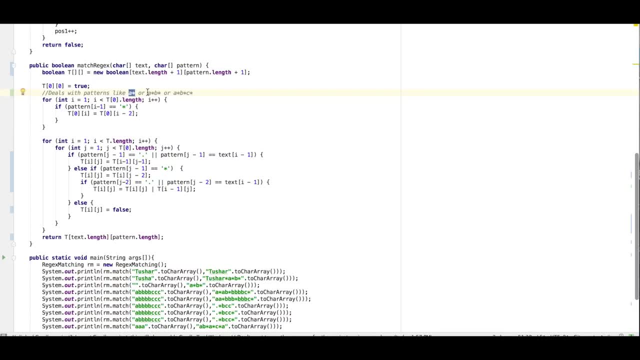 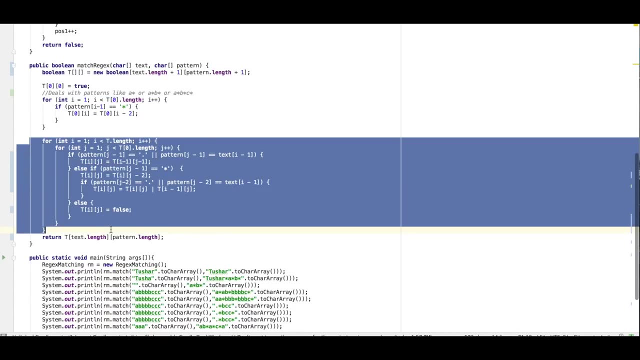 row. true if we have a pattern like a star or a star, b star, or a star b star, c star, something like that. So, after we are done doing all this, this is where the meat of the logic is. So our i starts from one and goes all the way till t dot length, and then j starts from. 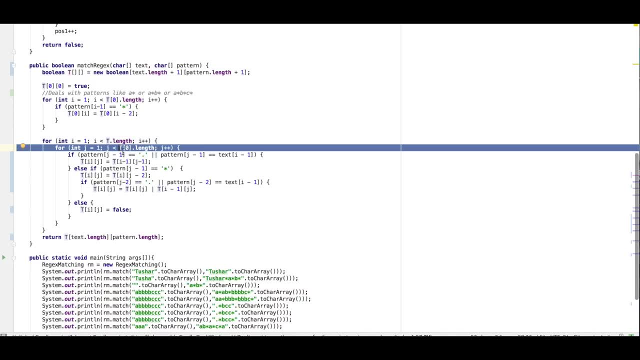 one and go all the way till t zero dot length plus one. And then, as we discussed before in the video, if pattern of j minus one is dot. So here Our pattern is a zeroth based index, which is why we are looking at the jth minus one. 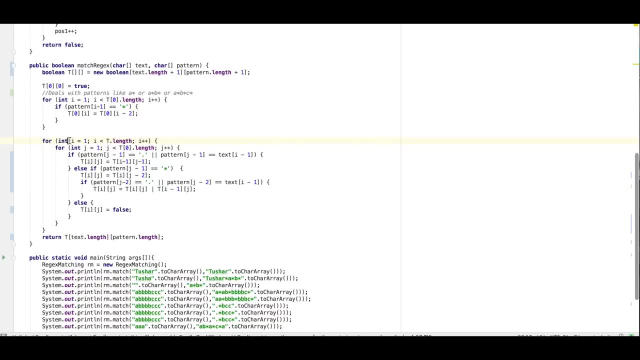 value and similarly for the text I'm looking for: i minus one value, because our i and j's are starting from one instead of zero. So if pattern of j minus one is dot, or if pattern of j minus one is text of i minus one, then t of i j becomes t of i minus one, j minus one. else, if pattern of j minus one, 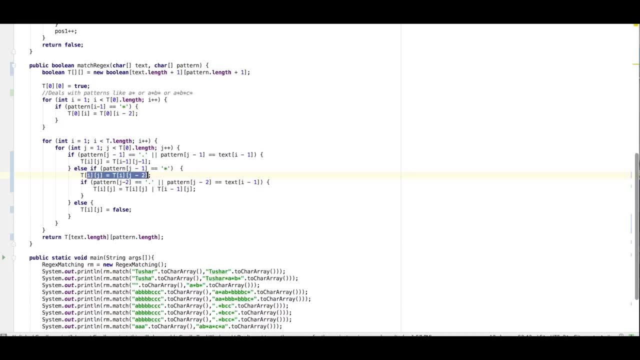 is star, then t of i j first becomes t of i j minus two. and if pattern of j minus two is dot or pattern of j minus two is text of i minus one- all this we discussed before in the video- then t of i j will be either whatever the value of t of i j is or t of.